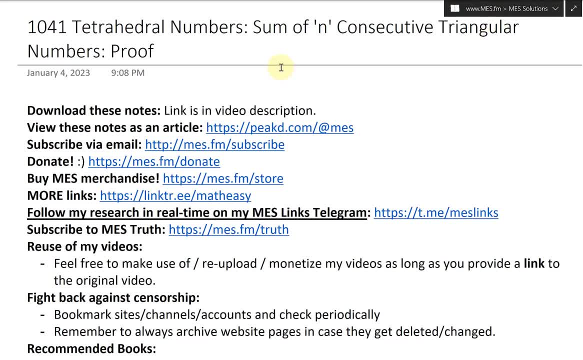 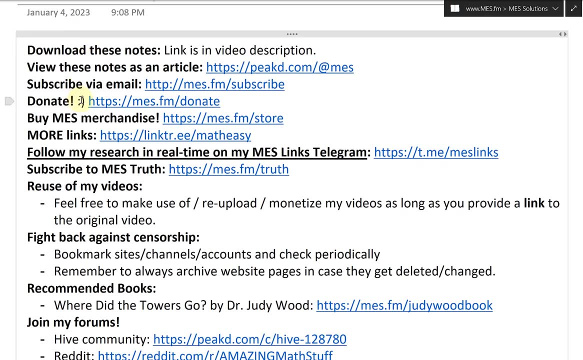 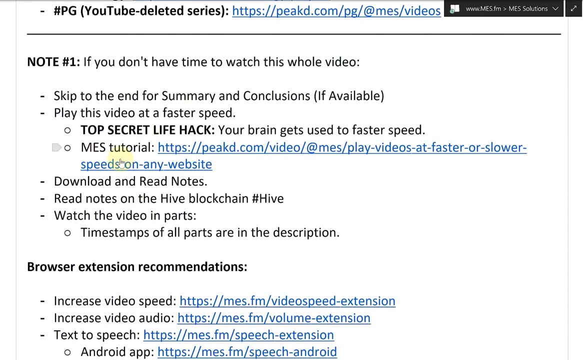 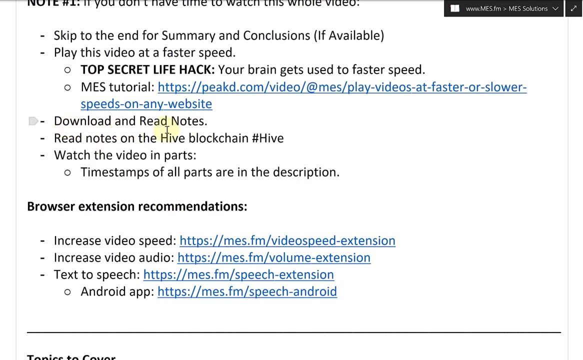 Hi, it's time for another math easy solution. Today we're going to go over a video on tetrahedral numbers, which are the sum of n consecutive triangular numbers, and then go over the proof of this. And yeah, interestingly, this video was a request that someone emailed me and, yeah, I thought I might as well go over it And let's jump right in. And before that, actually just a note: as always, if you don't have time to watch this whole video, you can play this video at a faster speed. You can also download and read the notes, or read the notes on the Hive blockchain, And, or you guys or you could watch the video in parts, and all the timestamps, as well as all these links, will be in the video description below, And you can even use a timestamp to skip even this intro, if you want. 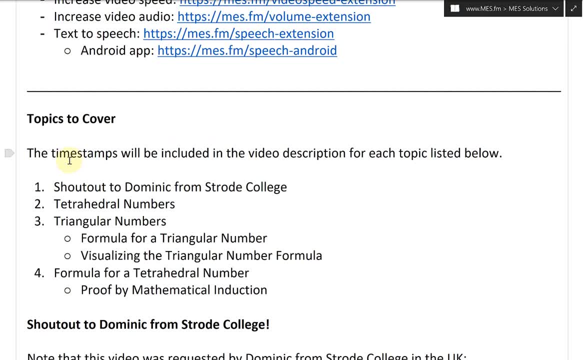 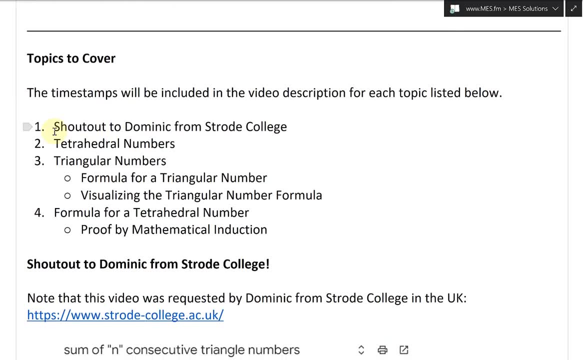 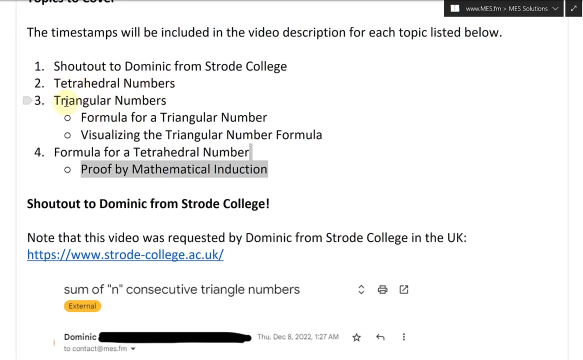 Anyways, let's jump right in. And so topics to cover And the time: yeah, note that the timestamps will be included in the video description for each topic listed below. And these are: yeah, these are the topics we'll cover. And then again, in the video description we'll have the timestamps. if you want to skip ahead and so on, So shout out to Dominic- Yeah, Dominic, from Strode College, He's the one that gave me the video request- And then tetrahedral numbers will go. then, after that, we'll go over triangular numbers and then formula for a triangle number, then visualizing the triangle number formula. 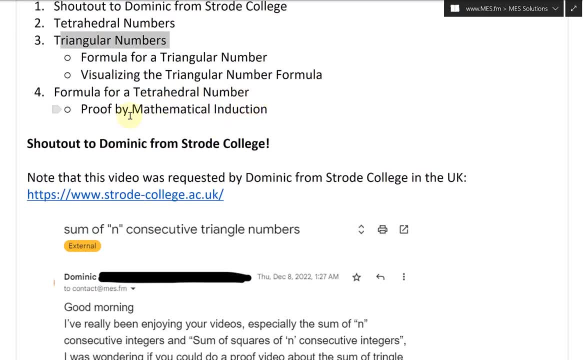 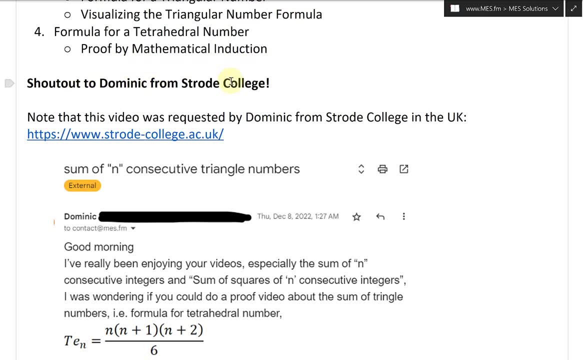 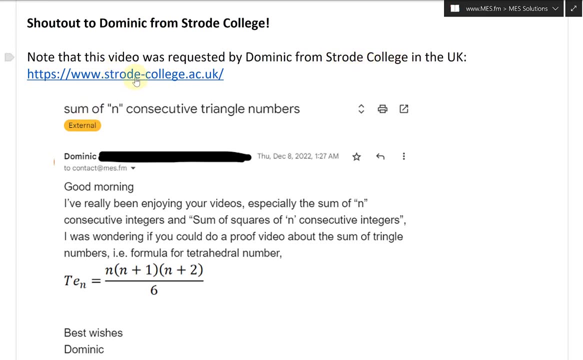 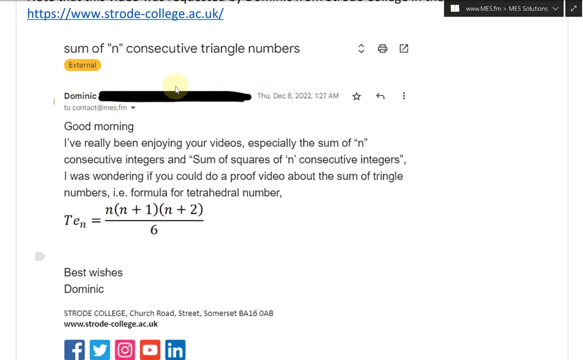 And then formula for a tetrahedral number and then proof by mathematical induction, And I'll just jump in. So yeah. so just a shout out to Dominic from Strode College. So note that this video was requested by Dominic from Strode College in the UK. Here's a link to the Strode College strode-collegeacuk. So his email is blocked out. his full name and email address. So some of n consecutive triangle triangle numbers: 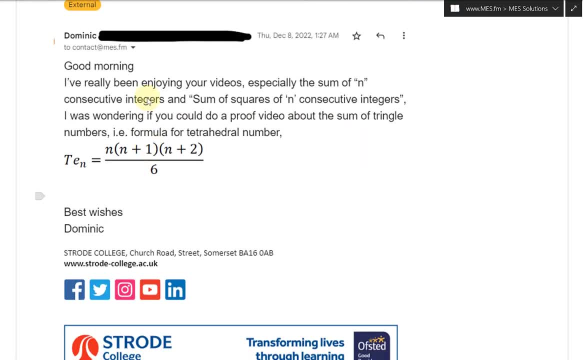 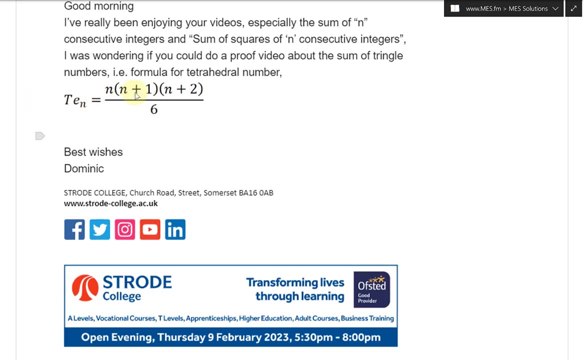 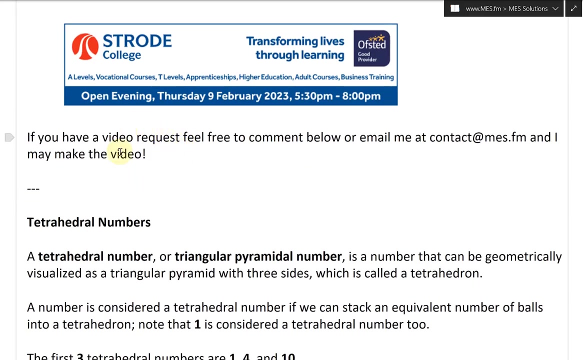 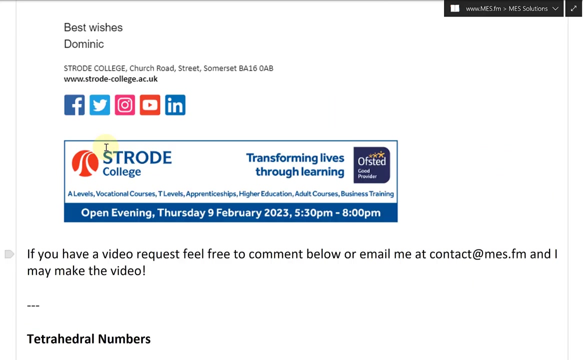 So yeah, good morning. I've been really enjoying your video, Especially the sum of n consecutive integers and sum of sum of squares of n consecutive integers. I was wondering if you could do a proof video about the sum of triangle numbers, a formula for a tetrahedral number. And this is the formula for a tetrahedral number. and then equals to n times n plus one times n plus one divided by six. And yes, from Dominic And I thought might as well go over it. So if you have a video request as well, feel free to comment below or email me at contact at mesfm And I may make the video if I can. 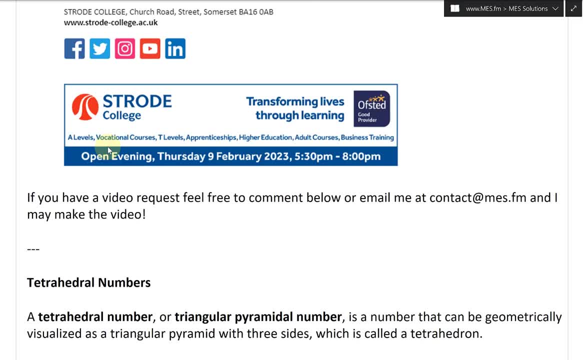 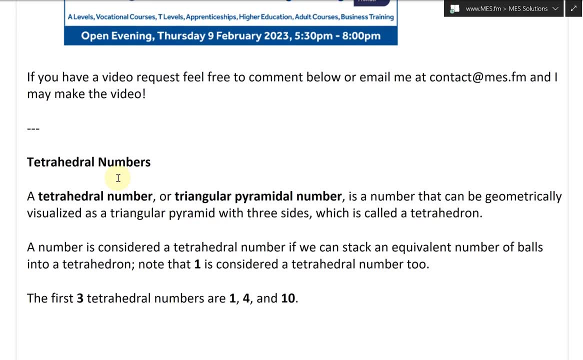 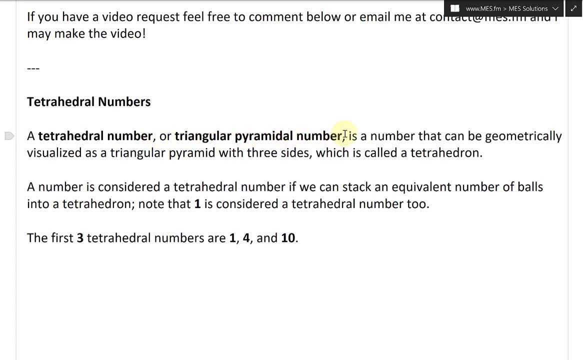 I think it's worthy. And, yeah, this tetrahedral number, I didn't hear, I didn't hear about this before And I thought it was pretty interesting And it is similar to my sum of n consecutive integers videos. Anyways, let's jump right in. So a tetrahedral number or triangular pyramidal number, Yeah, is a number that can be geometrically visualized as a triangular pyramid with three sides, which is this part is just called a tetrahedral And a number is considered a tetrahedral number, if we can. 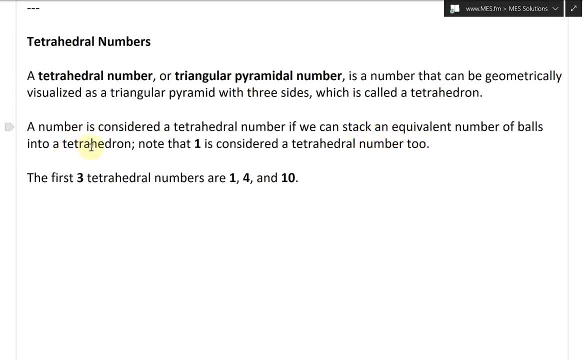 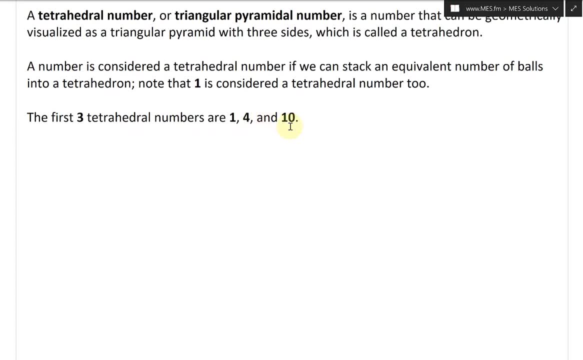 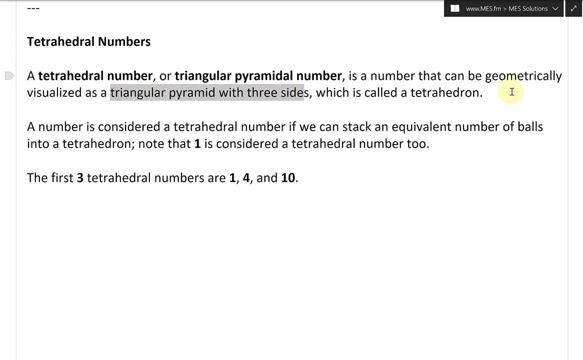 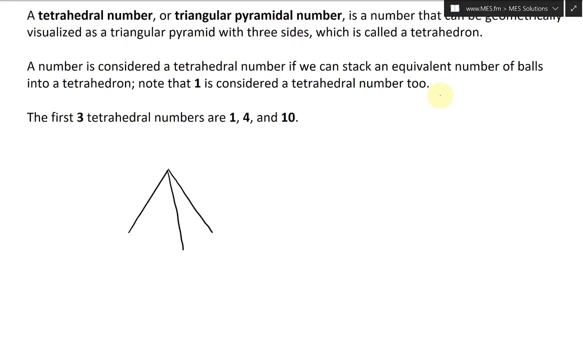 stack an equivalent number of balls into a tetrahedron. Note that one is considered a tetrahedral, number two And the first three tetrahedral numbers are one, four and 10.. All right, so let's just first draw this out. So let's just draw this triangular pyramid with three sides, In other words, a tetrahedron. So the three sided pyramid looks something like this, should be like this: All right, this is three sided pyramid. 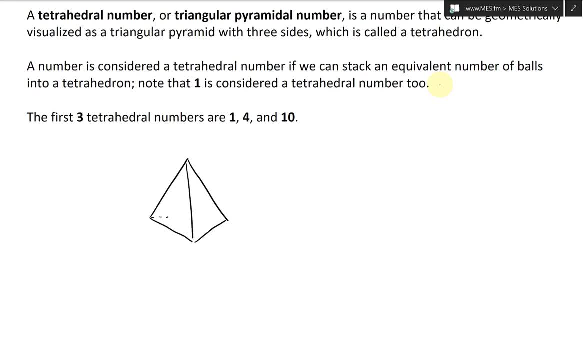 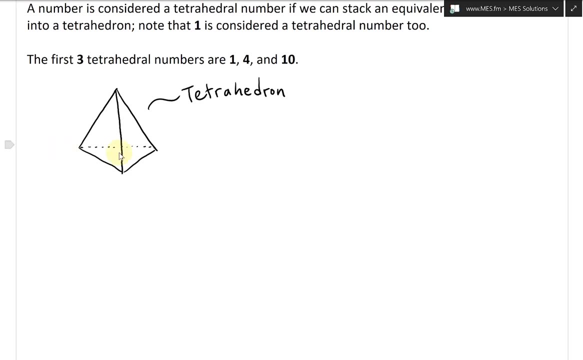 All right, here, I just fix that up. So three sides. let's draw the behind edge be dashed line across. So there's a three sided pyramid And this is again a tetrahedron. tetrahedron, All right here, I just moved it over here. So now let's write the first three tetrahedral numbers. One is considered a tetrahedral number on its own, So we'll just draw one here. There's, there's just one ball, is one like that? And now let's do the other side. 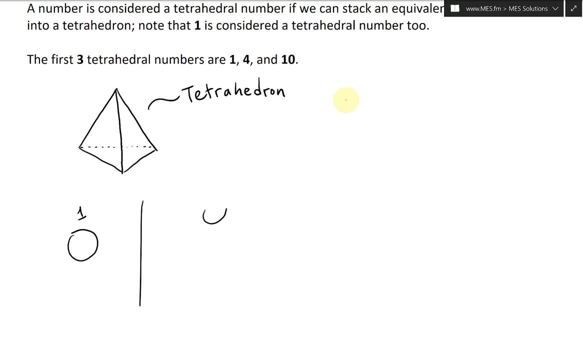 next one. the next one will have, let's say, one here, and if you put one on top of a triangular, uh, just a setup of balls, just so say three balls here, underneath one, two and then three, and then you stack them on top. let's say you have three balls like this, all right, so this is one here, so one. 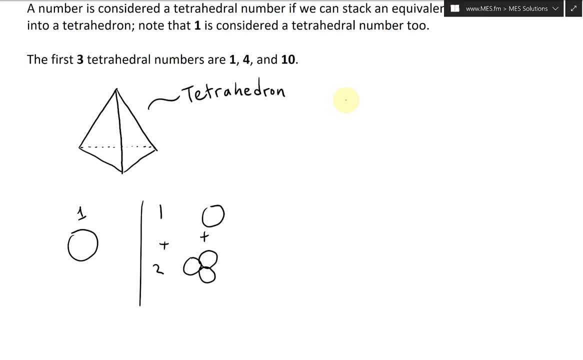 plus i also have this one plus this. three plus three, uh, this equals two. we're gonna have, well, four balls total and this is gonna be- uh, it's gonna- let's try this in 3d. so it's gonna be a ball on top ball here, then ball like this and then another ball in the background. so that's it so. 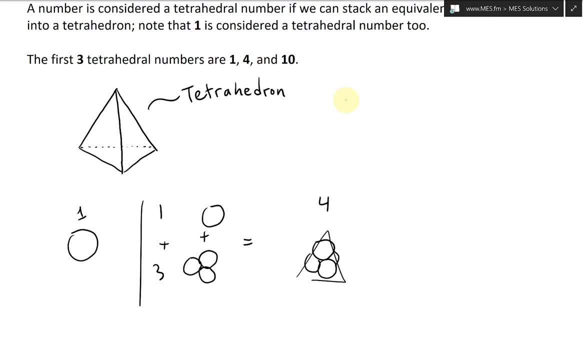 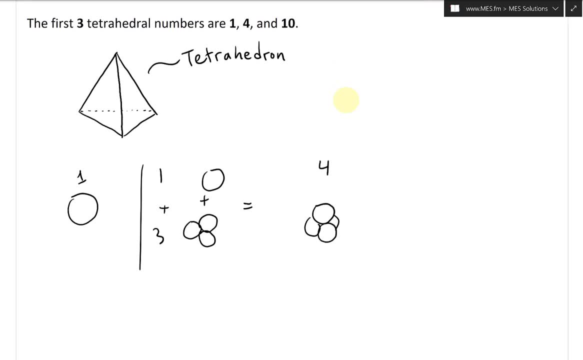 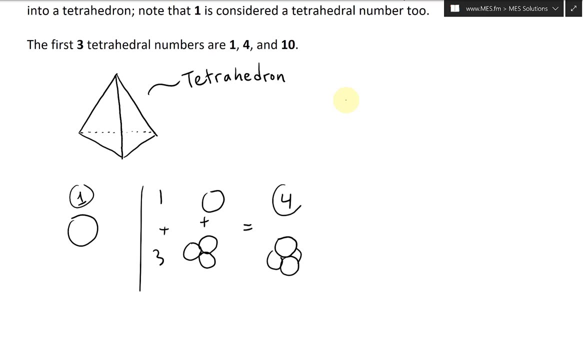 this is a stack of, uh, three pyramids, i mean three balls in a pyramid, triangular pyramid, etc. like that. i'll just ignore that and uh, yeah, so that's, that's gonna be our four. and uh, let's just put this all together here. so this is number four, so we have one four and then we have a three. 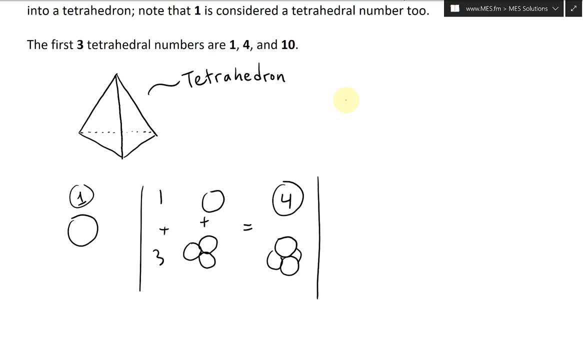 four, and then now the next one is ten. so we can see, that is well, we're gonna have one plus three, and then the next setup of uh triangles is gonna be, well, six. the next, uh biggest triangle, uh base. so we're gonna have uh- let's try this- in three. so we're gonna have uh one, which is this ball. 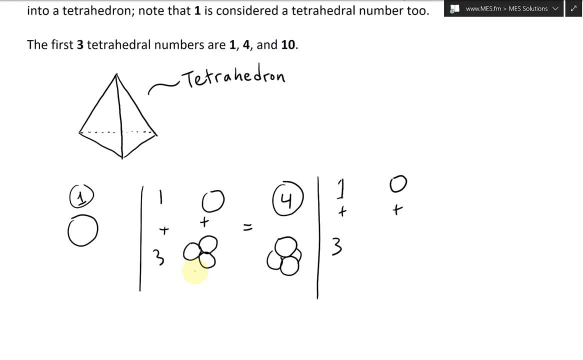 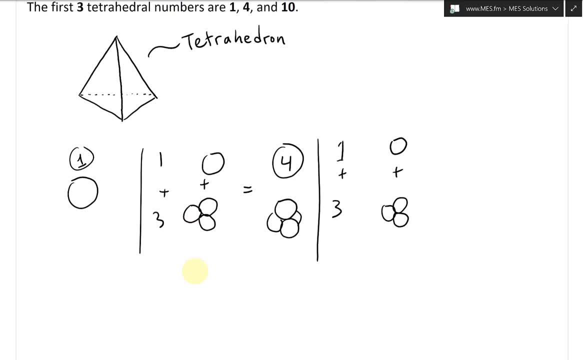 plus, and then plus this would be the three. so each time we're just adding another triangle or set up there like this: this is three, and then we're gonna have another plus, plus, it's gonna be six actually, and when you do that, it was well. see this here, now the 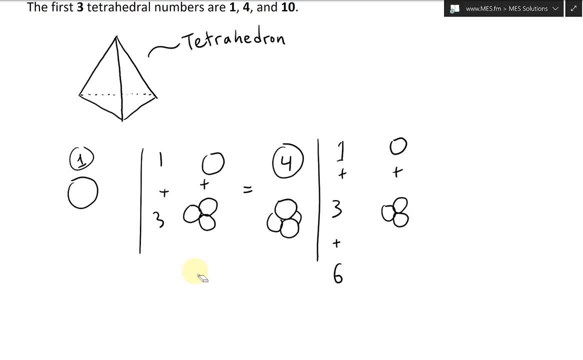 next biggest one is going to be added: one, two and three. so we're gonna, we're gonna have the three set up. here's one, two, three. then the next biggest one is going to be: well, we need another layer. so one, two and then three, so that's gonna be six total, and then this equals two. 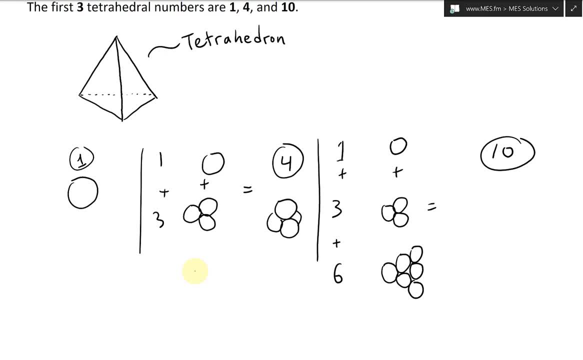 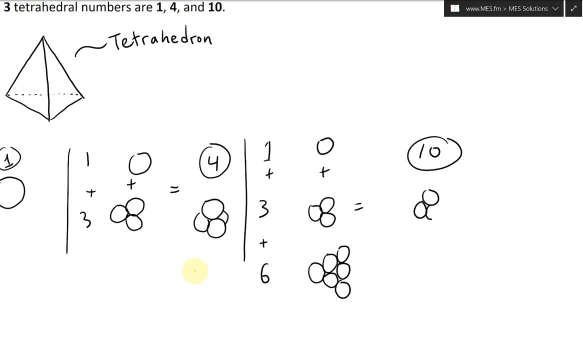 ten, the next number is ten, and this will look like, uh, just a pyramid balls set up, so one, we'll have another set up. i guess it's a bit hard to draw this- and that's three there. it's three on this, one, one on top, and let's draw this a bit better. 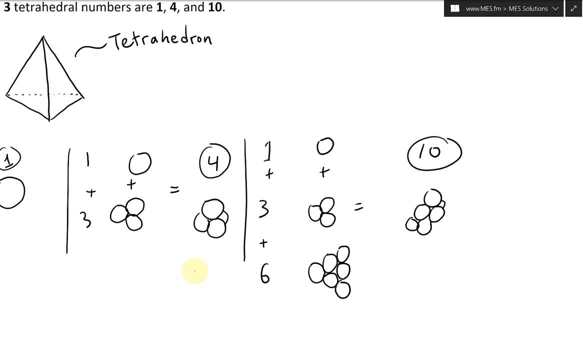 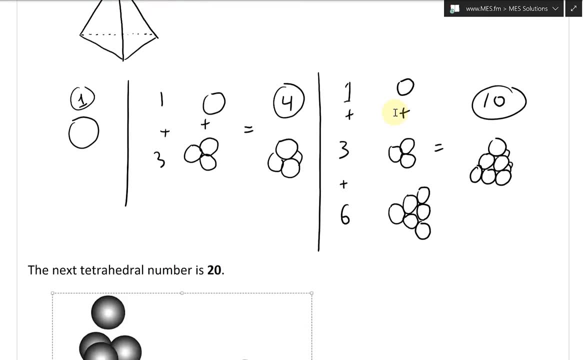 here. i just fixed that up, and now the next setup is: well, we're gonna have one here, one, and then three here, one, two. let's draw this. uh, all, right, now that we have all these, uh, tetradar number is one, four and ten. now the next one is: uh, well, it's going to be. 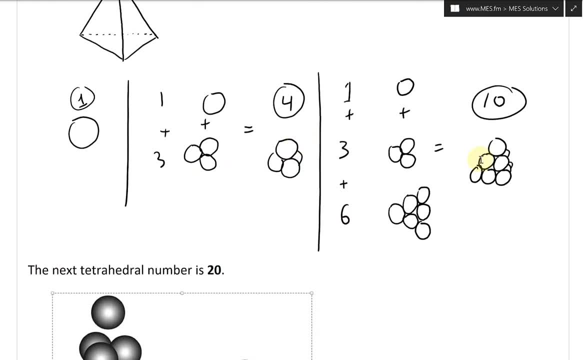 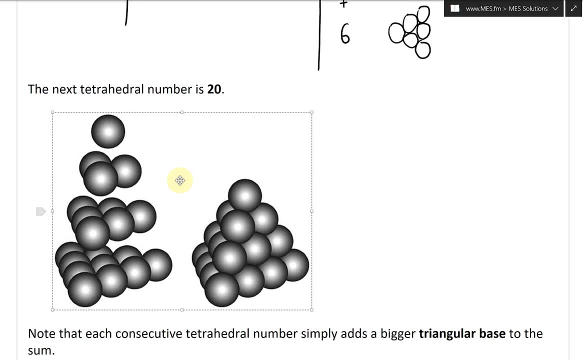 going to be here. the next tetrahedral number is 20 and i'm not going to draw, it's going to be too messy. but uh, basically you have the here, the same stack here. so notice, we had one, three, six, so we have a one here, and so we have a one here plus. now we have the three stack here, so one plus. 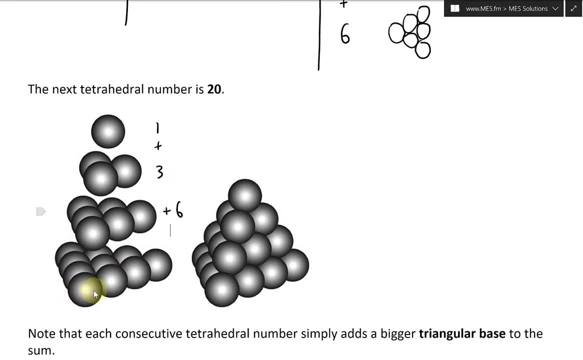 three and this other one's six, and that other one's going to be: well, we have four across here. so in other words, we just add another layer here, so it'll be six plus four. so this is one, two, three, four, five, six and plus four, so ten, and then this is going to be one, two, three, four, five, six, and 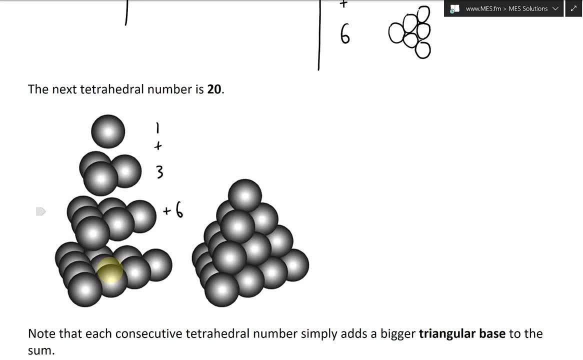 in plus 4,, so 10.. And then this is going to be well, 10. Plus 10. there Let's put a plus like this: Plus 6. Plus 10. And then this is going to be well. this previous one is: 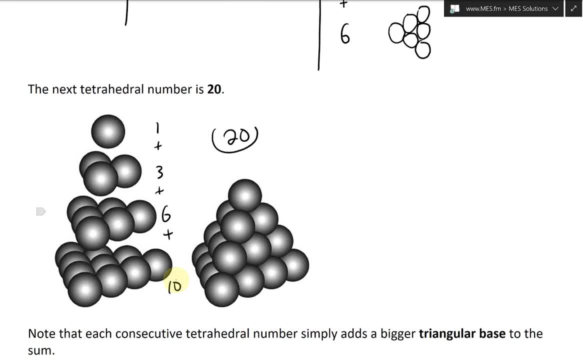 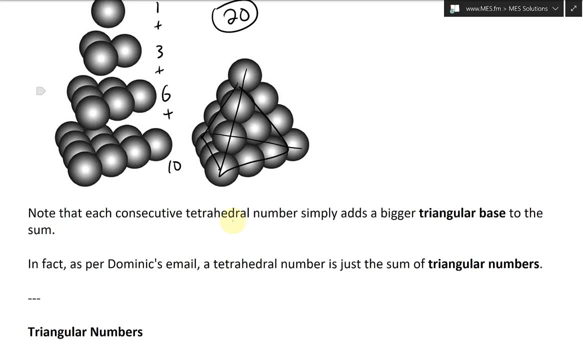 10.. Then we're adding another 10,, so this is 20.. So then the next one is 20. And you can see this pyramid there. So there's a giant tetrahedron pyramid like that And the background is going to be dashed like that. So that is a tetrahedral number, just so you could. 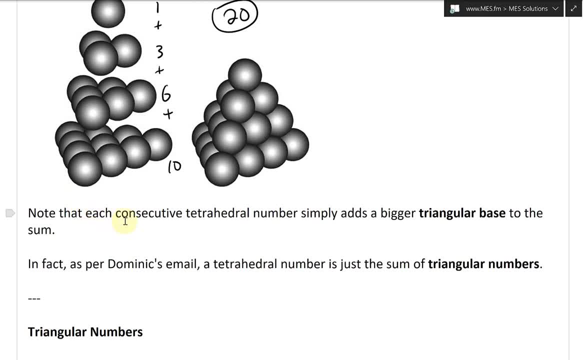 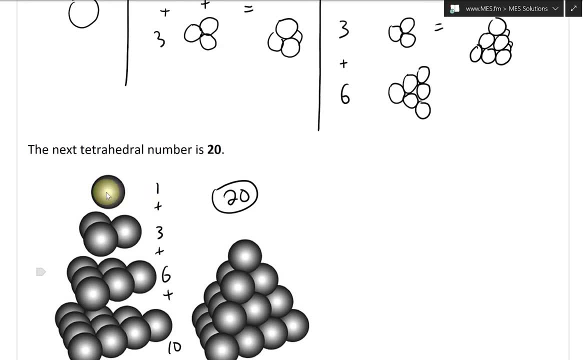 form a tetrahedron with stacking up balls, Anyway. so note that each consecutive tetrahedral number simply adds a bigger triangular base to the sum. So we add: here is 1. Then we add a 3 triangular base, Then we add a 6 triangular. 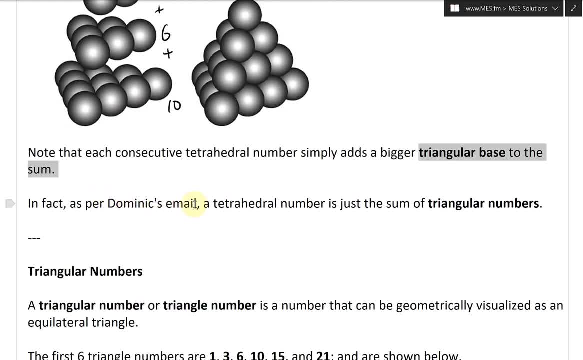 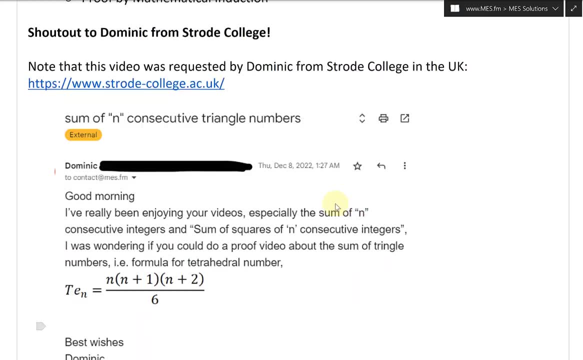 base and add a 10.. In fact, as per Dominic's email, a tetrahedral number is just the sum of triangular numbers. So in other words, as he says here. so right here is wondering if we could do a proof video about the sum of triangle numbers. 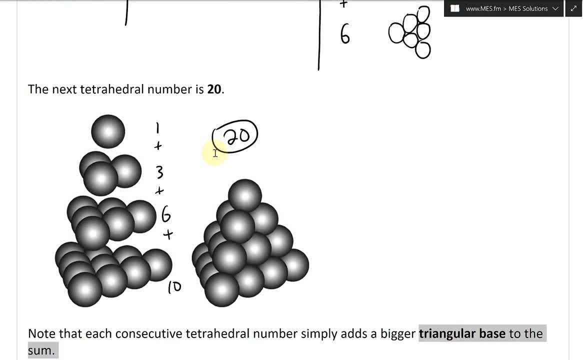 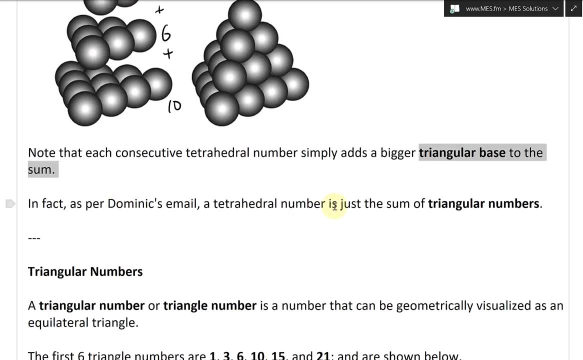 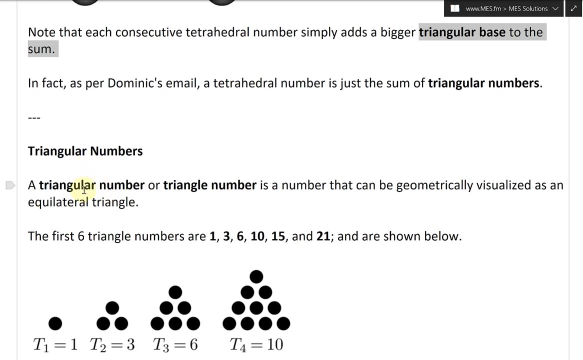 or triangular numbers, In other words formula of a tetrahedral number. So a tetrahedral number is the sum of consecutive triangular numbers. That's very interesting, All right. so that brings us to these triangular numbers. So a triangular number or triangle number? 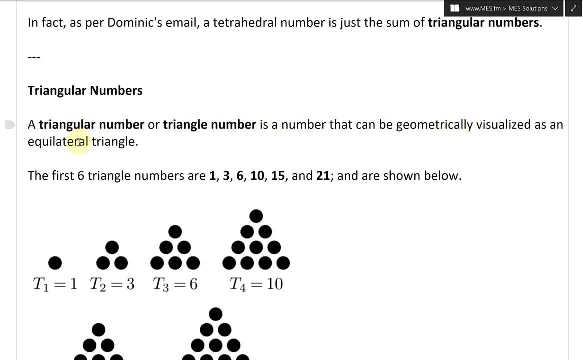 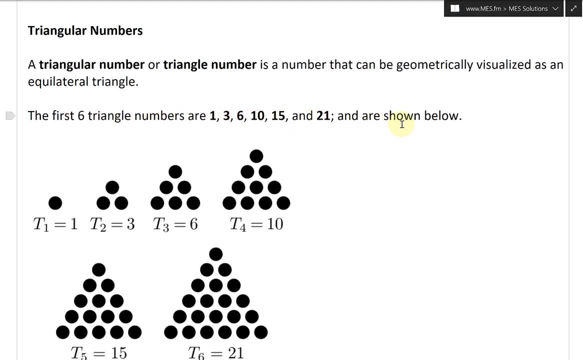 is a number that can be geometrically visualized as an equilateral triangle, And the first triangular number is a 1,, 3,, 6,, 10,, 15,, 21,, and are shown below. So you have: T is 1 there. 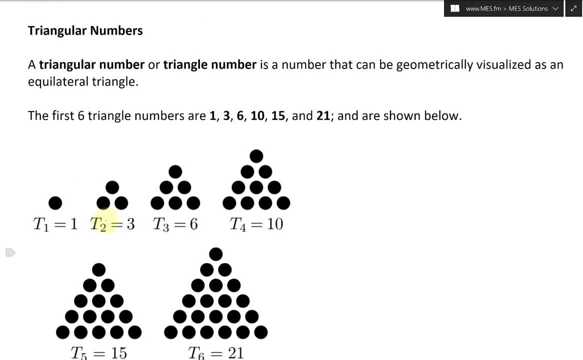 and T is. 2 is 3.. So notice, here we just add: if this is a 1, so this is 1 here, 1 here, then we have a 2 here, then we have 2 across here And the next one is going to be T is. 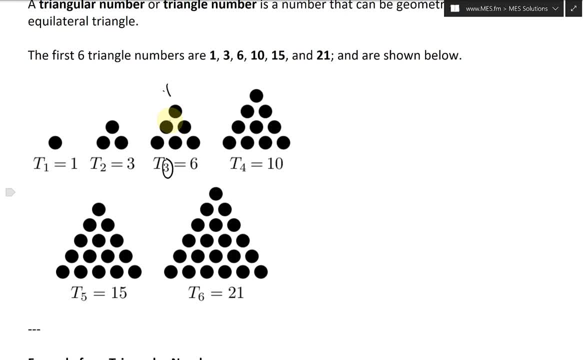 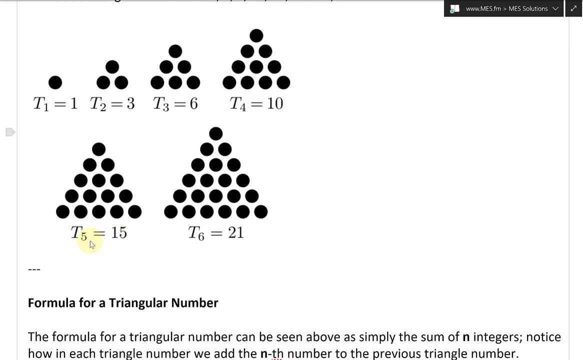 3, it's going to be 6.. We just add another 3 to this one here. So this is 3, adds 3, it's going to be 6.. And the next one, we add: well, 4, it's going to be 10.. And then T5. 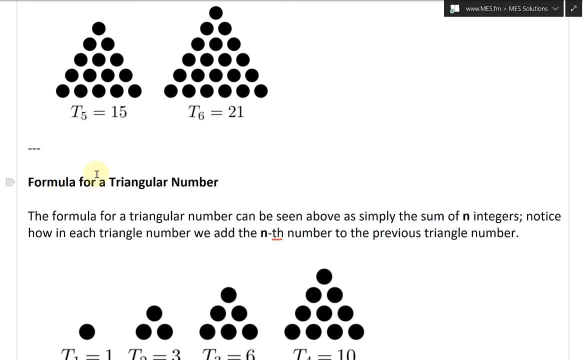 is 15,, T6 is 21,, et cetera. So formula for a triangular number- And yeah, the formula for a triangle number- can be seen above as simply the sum of n integers. And yes, as a sum of n integers, because, notice, here we're always adding, so this is a 1, then 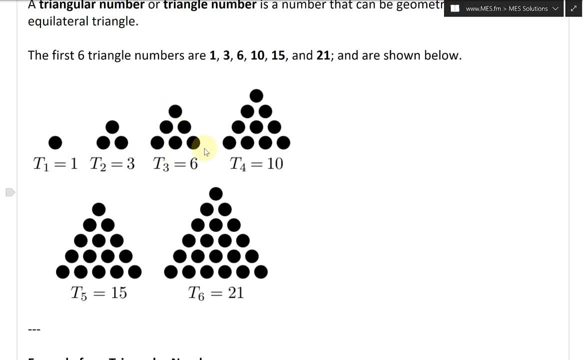 the next one, we're going to add a 2.. This is a 2 here. the next one, we add a 3, and we get 6,, et cetera. So notice how in each triangle number we add the nth number to. 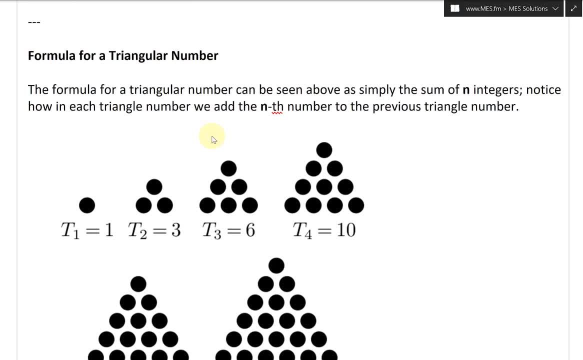 the previous triangle number, So in this one above here, as I was drawing it, but here I'll draw it. I'll draw it in just a better detail here. So we have a 1 here and there's a 1.. So that's. 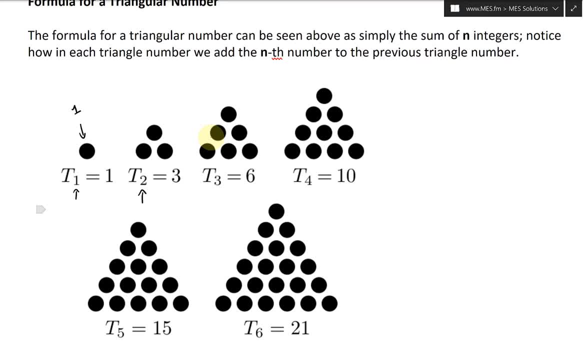 a 1.. Here's a 2, and we add to the previous one. So this is 1 there, and we're going to add 2.. And now this one here is 3, we're going to add 3.. Next one is T4, we're going to add. 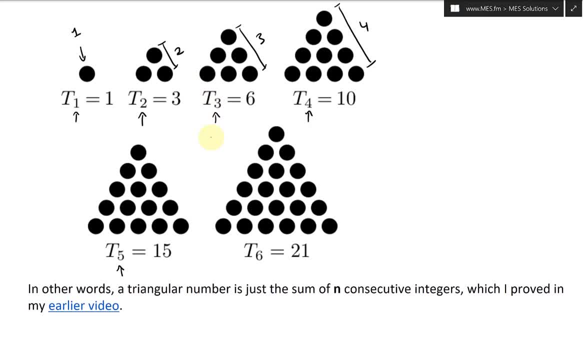 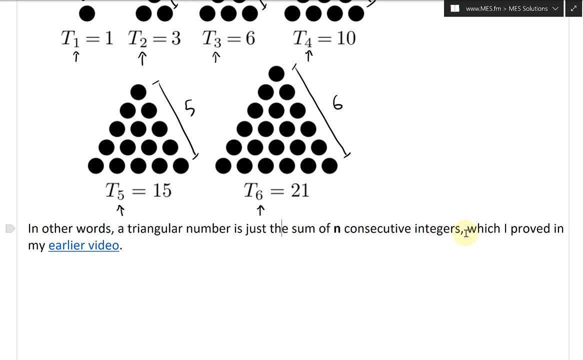 4.. Next one is T5, just for completeness, And then we're going to add 5.. The next one is 6, we're going to add 6,, like that, And in other words, a triangular number is just the sum of n consecutive integers, which. 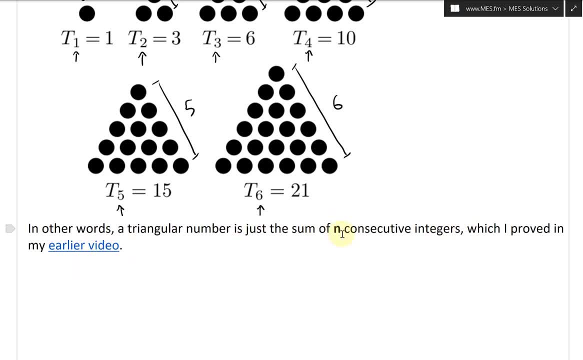 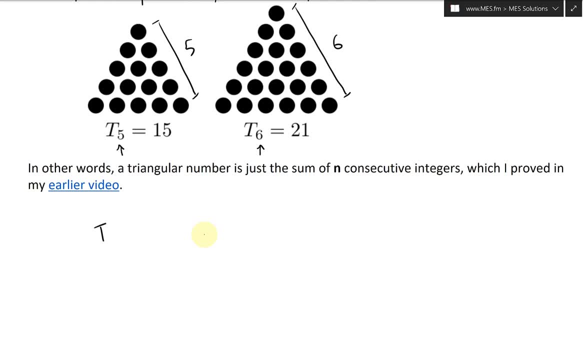 I proved in my earlier video on the sum of n consecutive integers, as Dominic references as well. So in other words, we'll call this triangle the number T, So Tn is just going to equal 2, but we have 1, then plus 2,, plus 3,, plus 4, et cetera, all the way to n. So 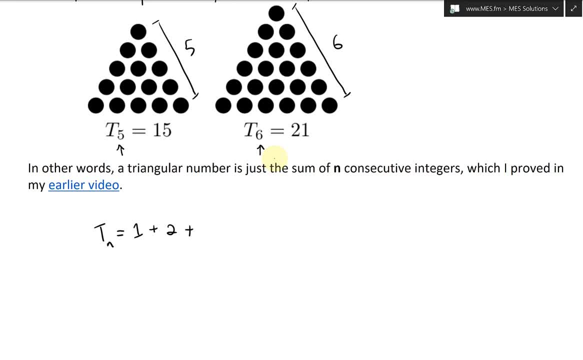 equals to 1. Plus 2. Plus 3. Plus 3. Plus 3, plus dot dot dot all the way to n. And this is equal to, as I proved in this video, is just going to equal to n times n plus 1.. You could see the video for the proof. 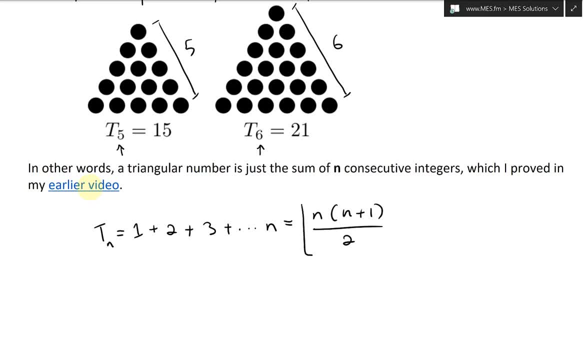 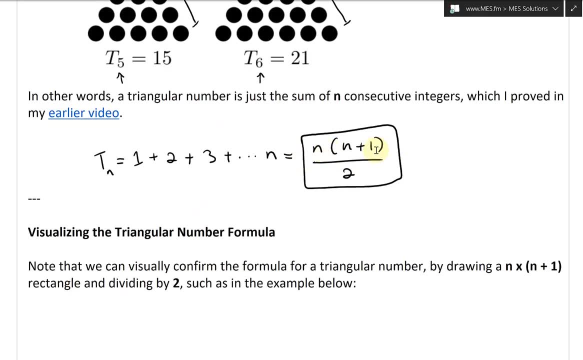 of it like that. So that is a triangular number. is this like that? All right, So now that we have this formula for this triangular number, and that's just a sum of n consecutive integers, we could also just visualize this formula. So visualizing: 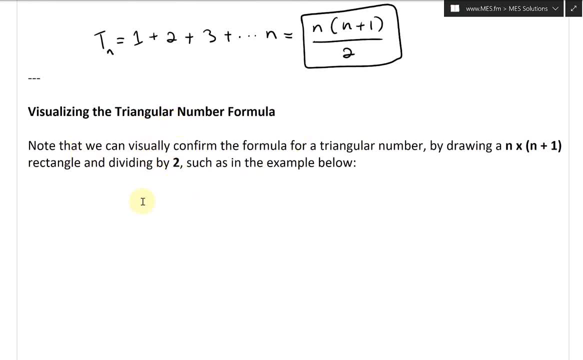 the triangular number formula And I didn't realize this before, so that's why I'm adding this here. pretty interesting, all right, so let's write this down. so note that we can visually confirm the formula for a triangular number by drawing an n by n plus one, a rectangle, and 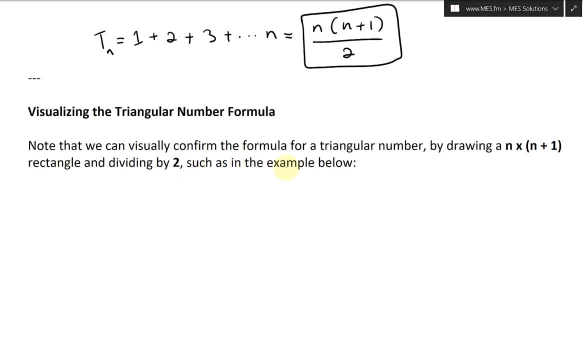 dividing by two, such as in the example below. so first let's write this: t4. let's take the fourth triangle number. this equals two. well, n is four, so we go four and then times it by n plus one, is four plus one this equal, and then divide by two, and then what we could do is: well, this is. 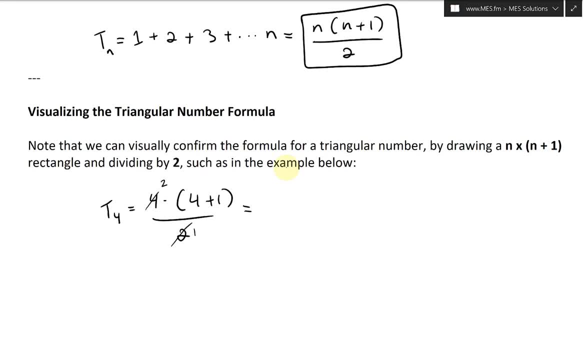 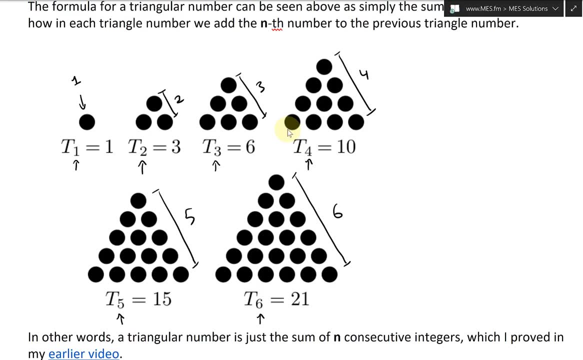 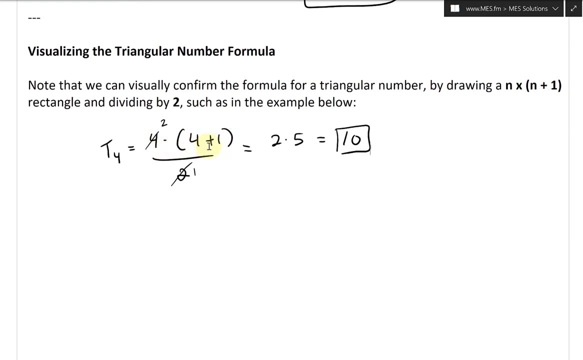 equals to. let's cancel this has become two. divided by that goes one. this equals to two times four plus one is five, which equals to ten. all right, so the fourth one is ten, as per here. so t4 is equal to ten, and we could visualize this formula as well: four times four plus one. 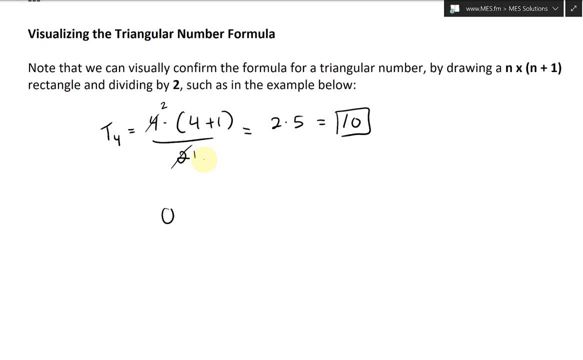 divided by two, and we'll draw this out as here. i'm going to do this, here i'm going to go, yeah, i'm going to go here. zero, i'm going to draw a ball, four balls here, and this is going to be: uh n is four. 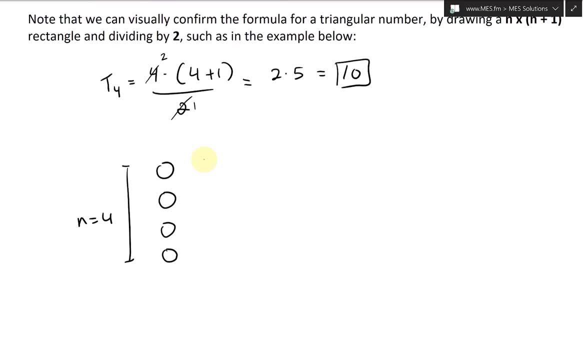 four, and then what I'll do is it goes all the way across here, zero. let's keep going. one, two, three, four. so we have four there, but instead of going to four, we want to go to this four times this, or this n times n plus one. so we're gonna. 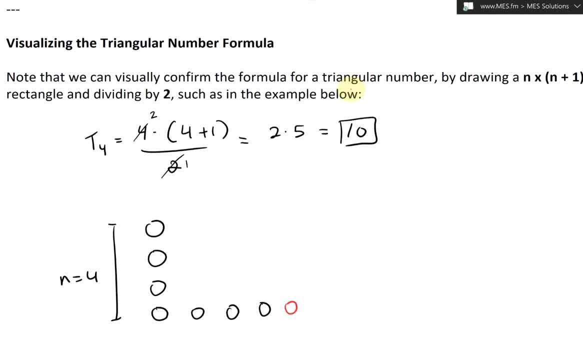 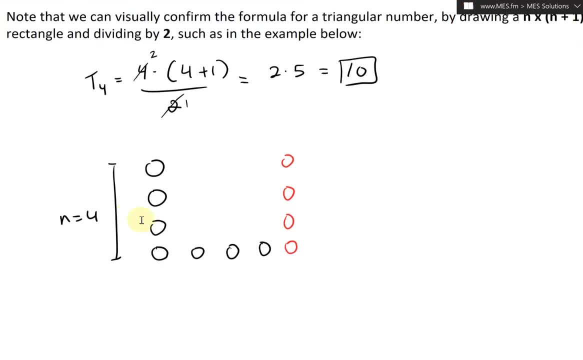 go one more, and I'll draw this in red: it's going to divide by two. so so now we have this, because it goes up like this, goes up and four like that, so we have a four by five, and then I'll draw another, set up here two, three and so on, and just 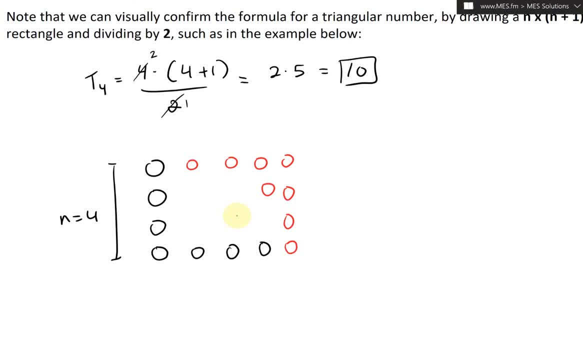 fill in all the blanks here. it's gonna match up with that. this one is gonna be here. that's gonna be there. it's gonna be another one here, another one here, another one there. now, let's change the other colors. get back here. so that is actually. this one is wrong. this is gonna be black. 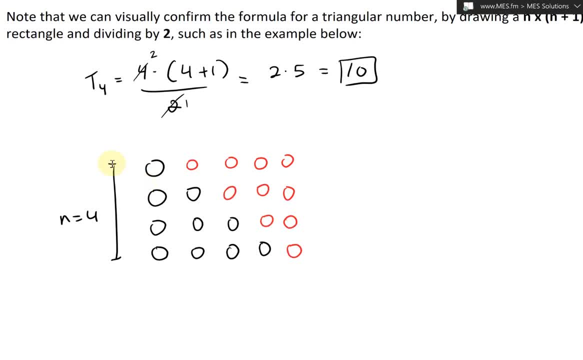 yeah, so now we have exactly exactly two things have. so that's a: n equals four- this is gonna be up to here- and equals two. I'm just n plus one. n plus one is equal to five, like that. and then the triangle number is: we take this and just divide by two, so we're gonna. 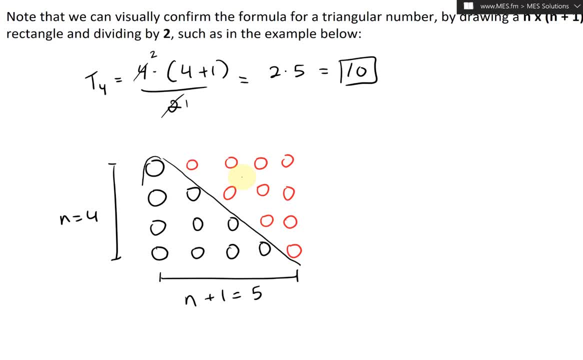 have, yes, set up like that. so now we have divide by two and now we we have this triangle number. so there's a triangle number there and there's a triangle number across here. so we divide that into two and we have two triangle numbers and this one's gonna be ten. so you get a one, two, three, four, five, six, seven, eight. 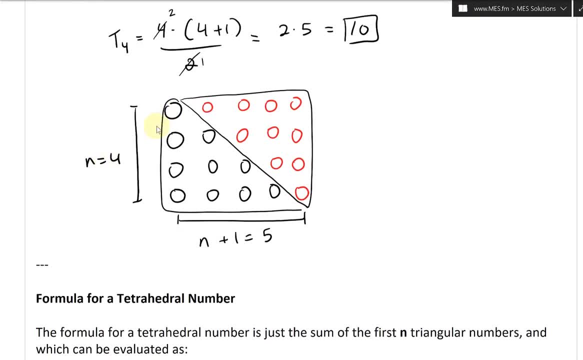 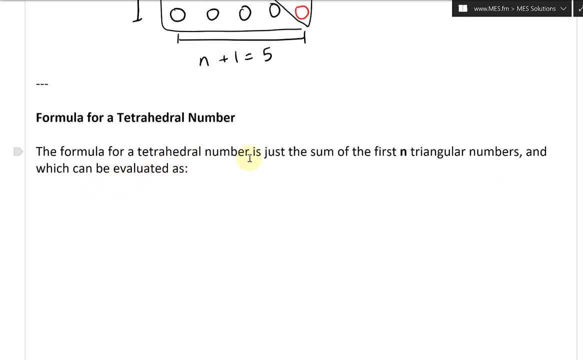 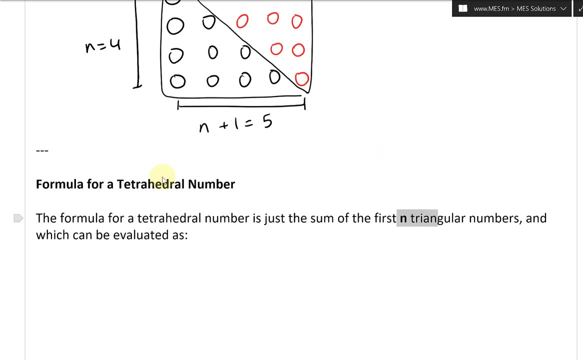 nine, ten. so yes, epic stuff. all right. so now that we covered triangle numbers, and now let's look at formula for a tetrahedral number. so the formula for a tetrahedral number is just the sum of the first and triangular numbers which can be evaluated as. so again, remember, these are just triangle numbers and then 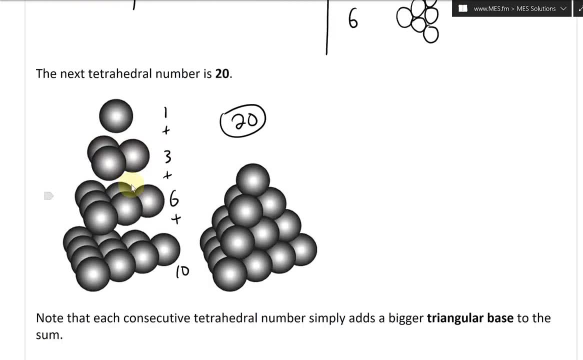 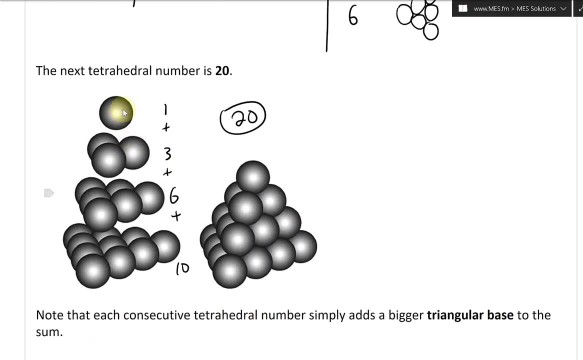 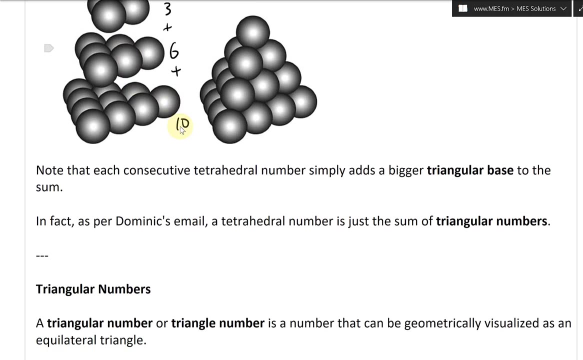 the, the tetrahedral numbers. you're adding all of those tetrahedral numbers as all those triangle numbers. so the triangle numbers are just the sum of the integers and then these one are the sum of the actual triangles. so, in other words, we're taking the sum of the sum of integers and, yes, we're adding each one. 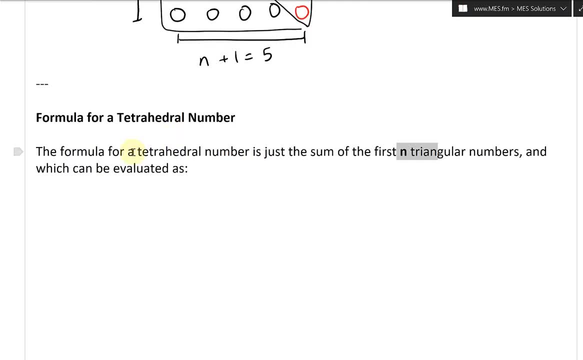 there to it. so pretty epic stuff there. so the formula for a tetrahedral number is- and it's gonna be right like this: T. you will call this TE for tetra, for t, tetrahedral. and then the nth tetrahedral number is equal to the sum and. 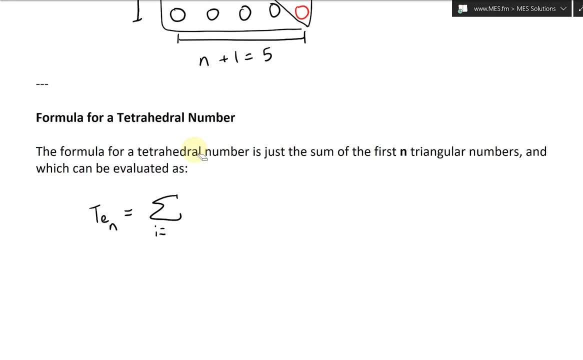 of, from I equals to, I'm gonna, let's go to K, from K equals to once when it started from the beginning, all the way to n, and so we're gonna sum up, and then we're gonna go T, K, so we're gonna sum up n of these triangle numbers, yeah, so we. 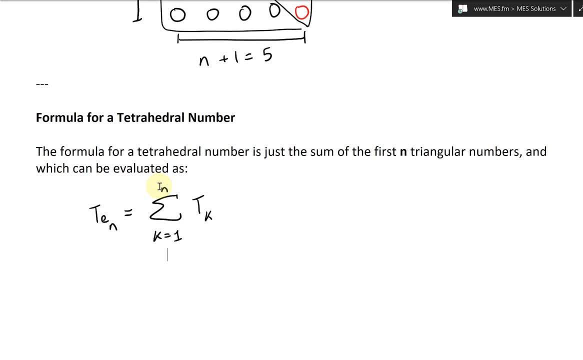 start off from K at T 1, T 2 plus T 3, all the way to T and or better yet. I'll smooth this over there and just write this for incompleteness. so this equals to the first triangle, number, T 1, plus the second, T 2, plus T 3, plus dot dot dot. 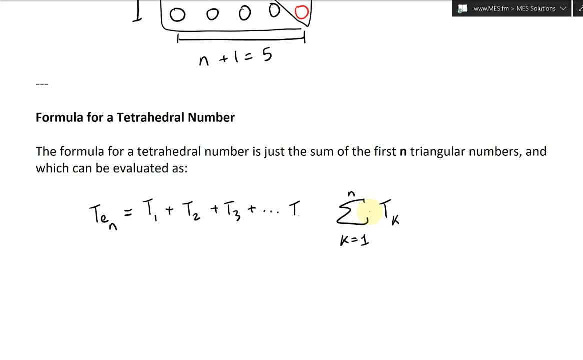 all the way till T, n, T sub n. so we're just adding all the triangle numbers to it and you could write that in summation format like that: the same thing is writing: T from starting from K equals 1 all the way to n of T, K, so of the. 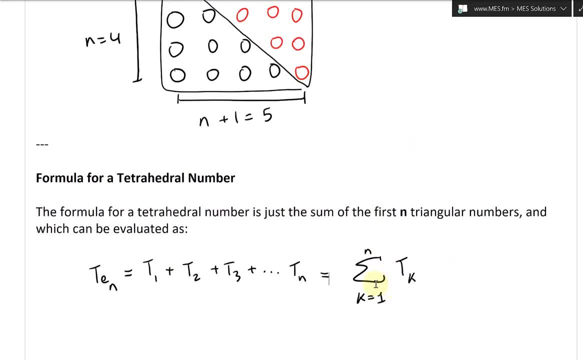 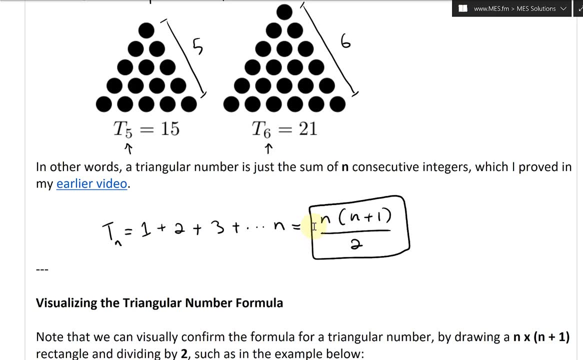 triangle numbers like that. alright, and, and we know the formula for the triangle number there that is just the: yeah, that's just the sum of n consecutive integers. and here I didn't write it in the format, the summation format. just move this over here. this equals to summation from: I equals to 1 up to. let's go up to n. let's go up to n. 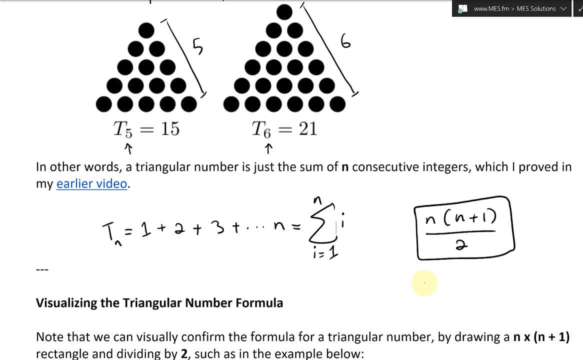 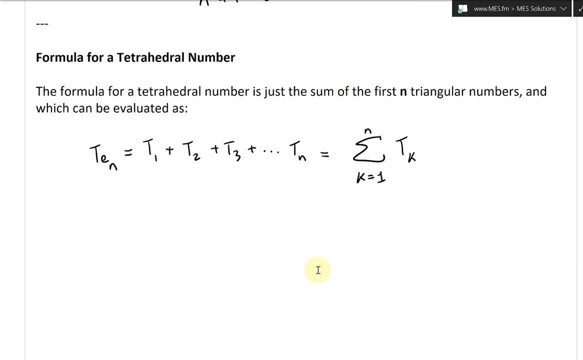 and this would just be of I, so that's integer. I for integer, so I is 1, then 2 and 3, all the way until n. this equals to this formula right here. alright, so that is what we have. let's scroll down here. so this equals 2. yeah, 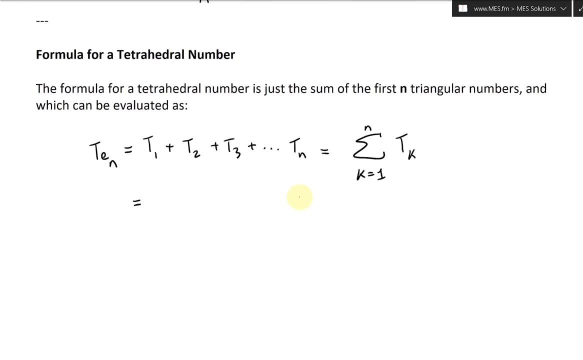 this equals 2, and let's just write it down over here. this equals to the summation of: from K equals to 1, all the way up to n of. and now this T, K is a summation itself of integers, so put a bracket summation this is gonna be up to. 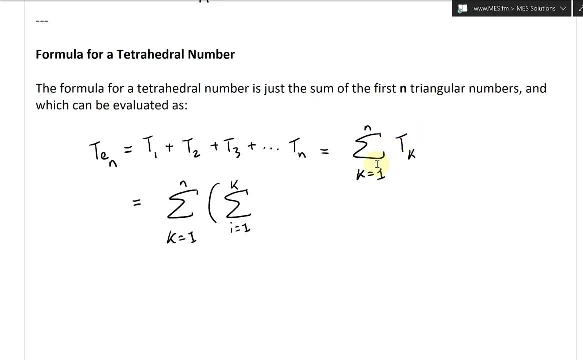 K now from I equals to 1 up to K, because we already have a n here, so just use K and this is gonna be of the integer. I like that. and now this equals to: and I was just just put in our formula for the n consecutive integers, this one right here. 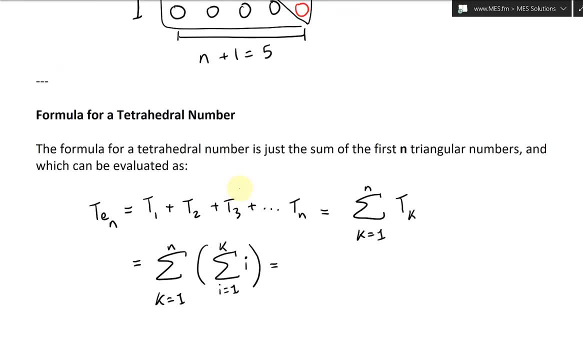 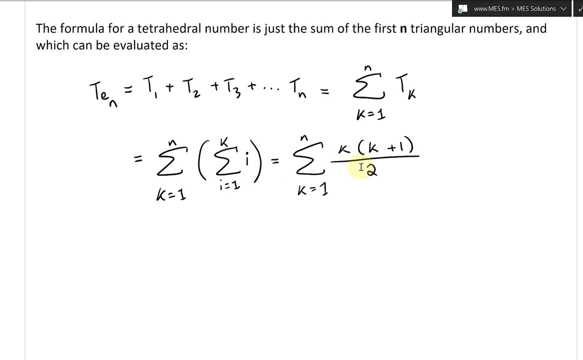 and times n plus 1, but in this case we're gonna have K. this equals to the summation up to n from K equals to 1 of K times K plus 1 divided by 2. yeah, I'm gonna, yet divided by 2, right here. I just fixed up everything right here and yeah. 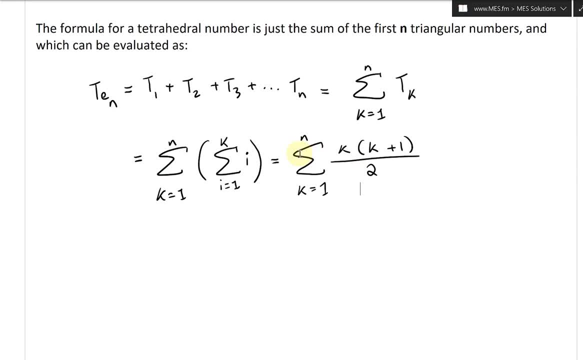 so this summation of these triangle numbers equals 2, and putting in the formula for that the consecutive integers, it's going to be well. summation from K goes to 1, up to n of K times K plus 1 divided by 2. and now, if you, 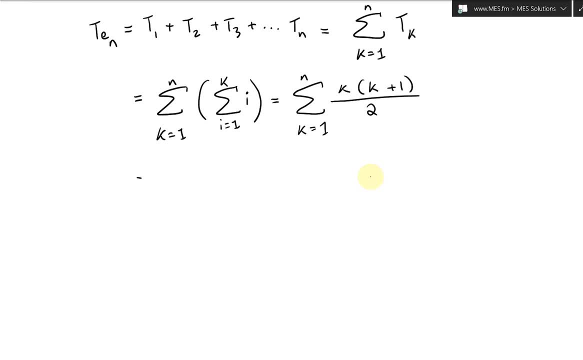 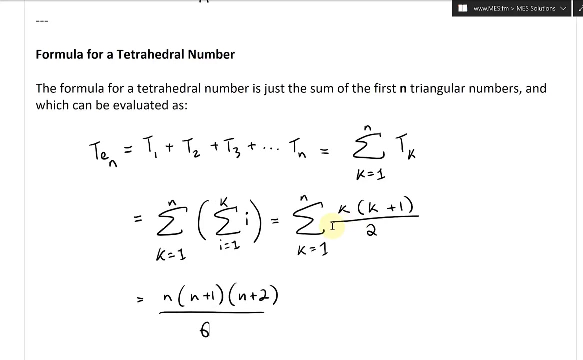 evaluate this, or or basically what this ends up becoming is, and we'll prove it soon- this equals to n times n plus 1. so the full summation times n plus 2, like that, all divide this by 6. so notice here of the sum of n integers. is K or, or just equals to well. 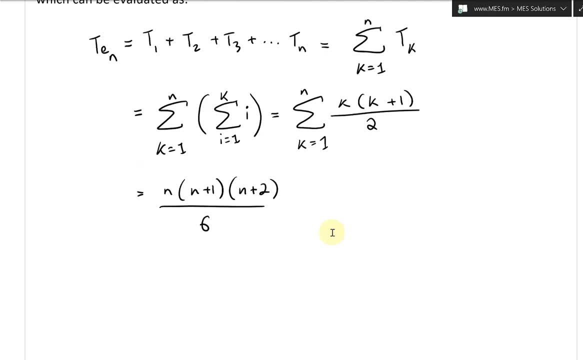 n times n plus 1 divided by 2, for triangle numbers is gonna be n times n plus 1, times n plus 2, and then divided by 6 as opposed to divided by dividing by 2, it's pretty epic. so I'll put this here and write T? en like that smooth. 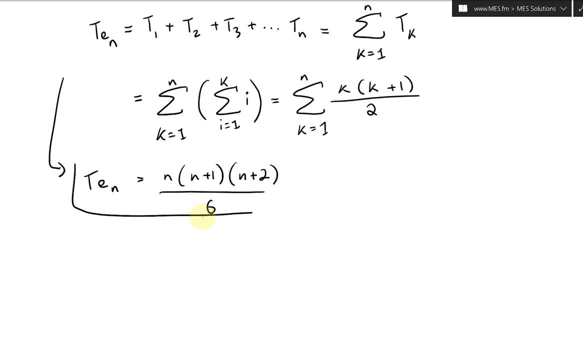 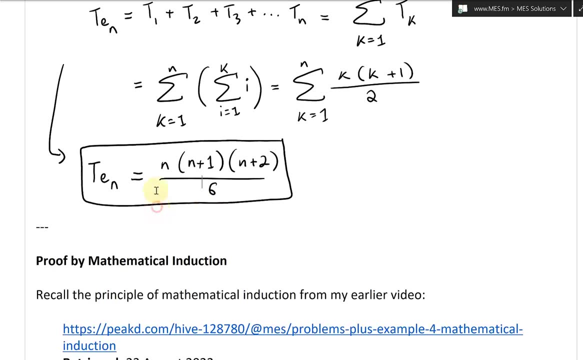 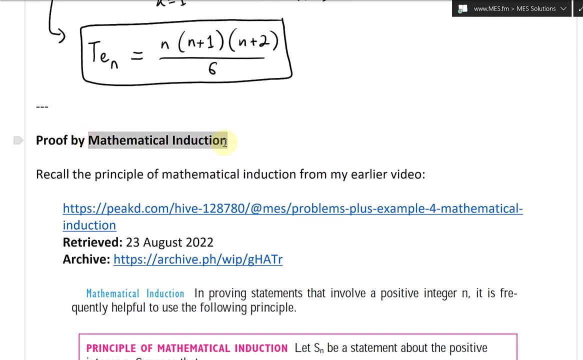 that this whole thing above here. so this equals to the formula for a, try, a tetrahedron number to remember, and I will prove this soon. all right, then then, now that we have this formula, now let's prove it, and we're gonna prove that by mathematical induction. so recall the principle of. 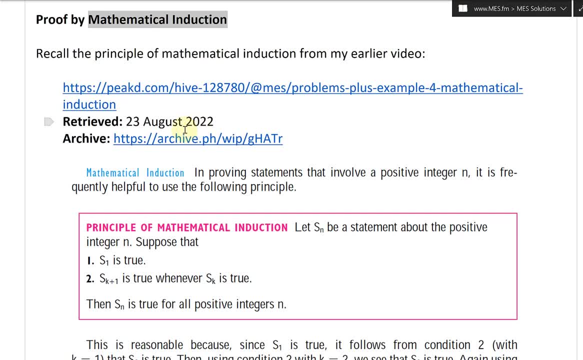 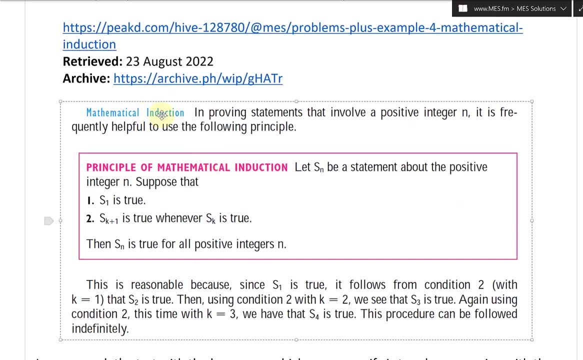 mathematical induction from my earlier video and now here's a link to the hive article on it and close the video link and so on, and then here just copy for my calculus books. just as neither so a mathematical induction improving statements that involve a positive integer, and it is frequently held. 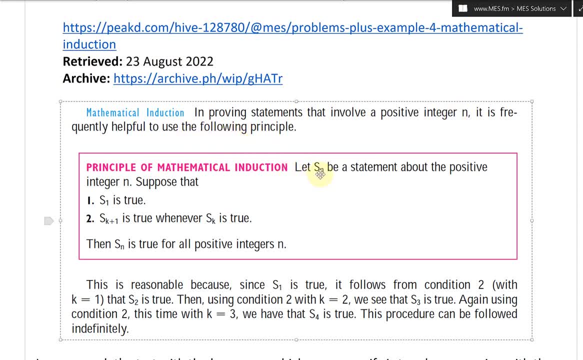 helpful to use the following principle. So let s n be a statement about the positive integer n. Suppose that s1 is true and that sk plus 1 is true. whenever sk is true, Then sn is true for all positive integers n. So, and this is reasonable, because since s1 is true, it follows from condition. 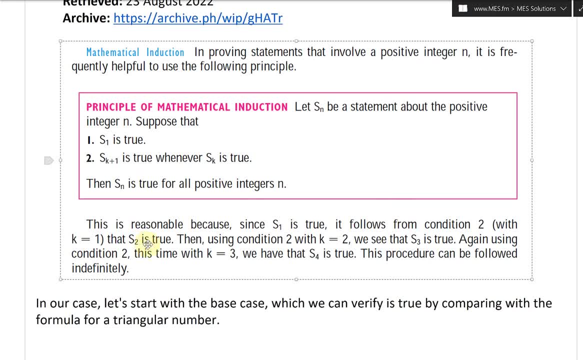 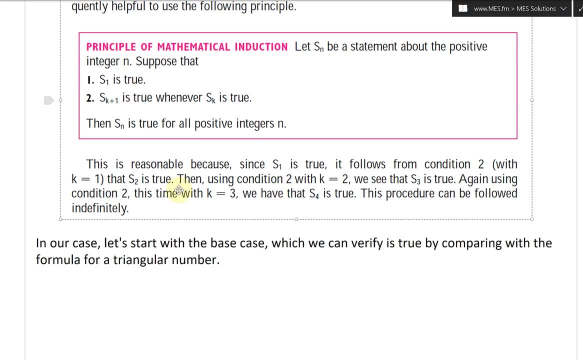 2 with k equals 1, that that s2 is true. Then, using condition 2 with k equals 2, we see that s3 is true. and again using the condition 2, this time with k equals 3, we have s4 is true. This. 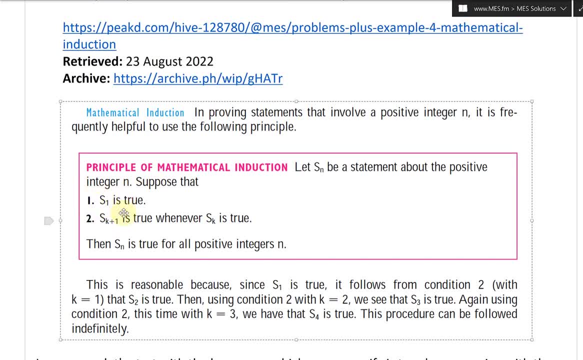 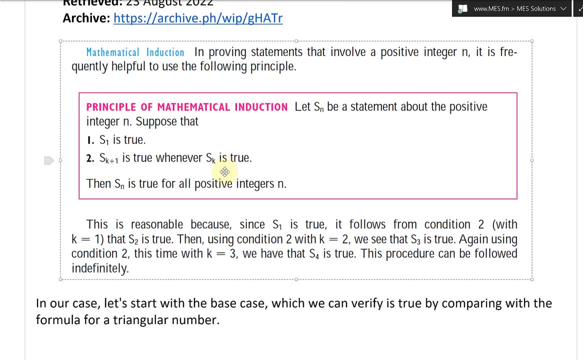 procedure can be followed indefinitely. So, basically, all you got to do is prove that. well, yeah, show that s1 is true and then show that sk plus 1 is true whenever this is true, because once you once s1 is true, s2 will be s3, etc. So in our case, let's start with a base case or another. 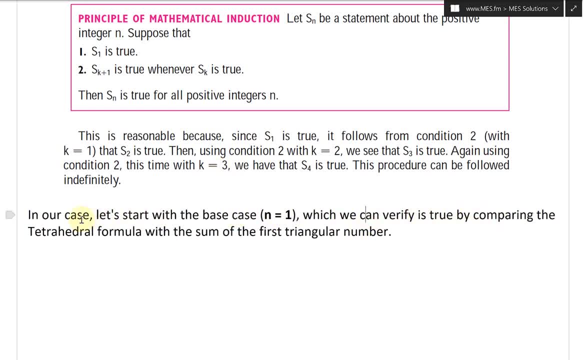 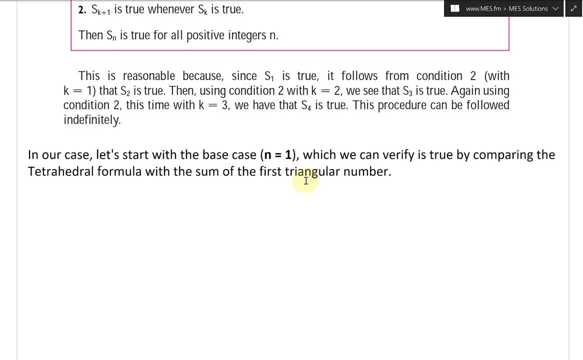 the words n equals 1, which we can verify is true by comparing the tetrahedral formula with the sum of the first triangle number, because, again, that's what just a tetrahedral number is. So the base case n equals 1, that's just going to be well. again, that's just going to be 1.. So the answer: 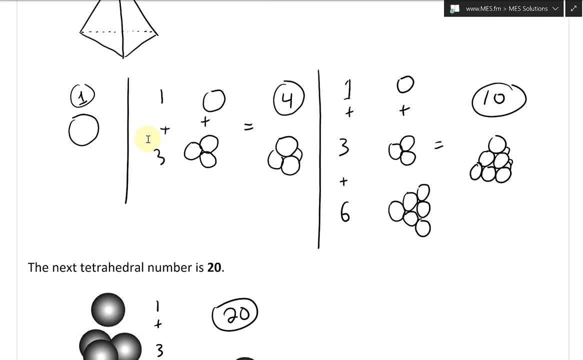 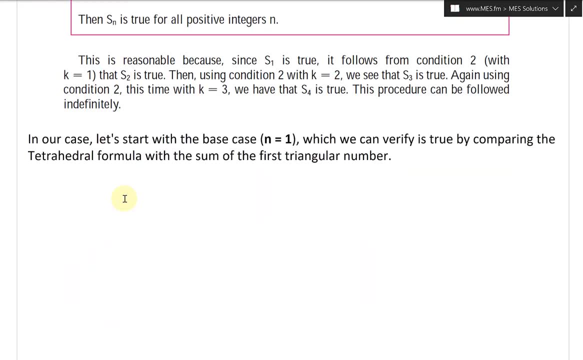 should be 1 here. that's the first case. and yeah, let's just sum it up. And the first triangle number is just 1, so both of them should be 1.. So let's write this out. So in this formula is: 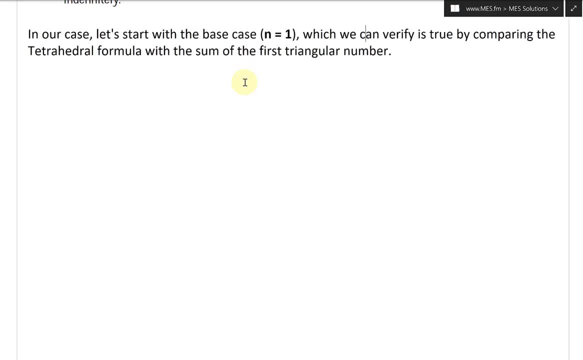 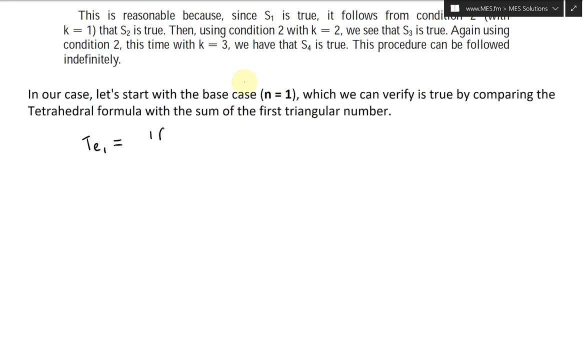 n times n plus 1 times n plus 2, divided by 6.. So Te1 is equal to n, which is 1, times 1 plus 1, n plus 1, times 1 plus 2, which is n plus 2,, and then divided by 6.. This equals 2, well, 1 times. 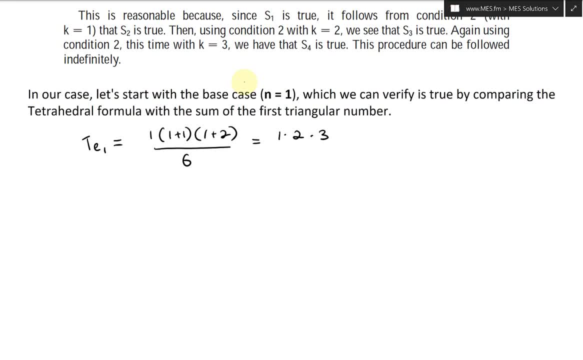 1 plus 1 is 2, and then 1 plus 2 is 3.. So 1 times 2 times 3, divided by 6, and that's just going to be 2 times 3- is 6.. 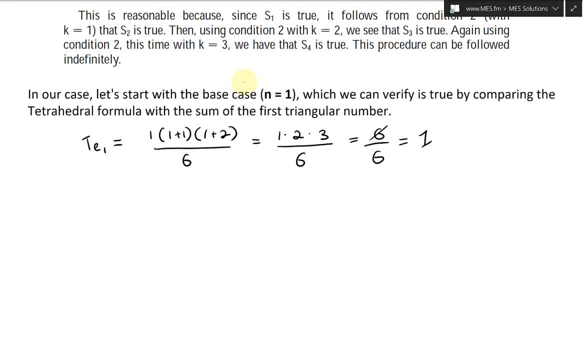 And then, divided by 6, equals to 1,, so they just cancel. All right, so this is 1, and that's, that's correct. We could also see that with the first triangle number, and then so Te1 is also equal to. well, just Te1, the first triangle number. And in writing this in summation format: 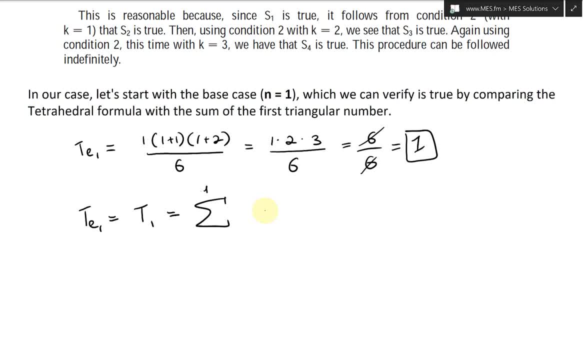 you could write this as: n equals 1,. let's put 1, up to, from k equals 1, all the way to 1,. this is going to be actually. I was going to write the summation, but I'll just skip it over to this. 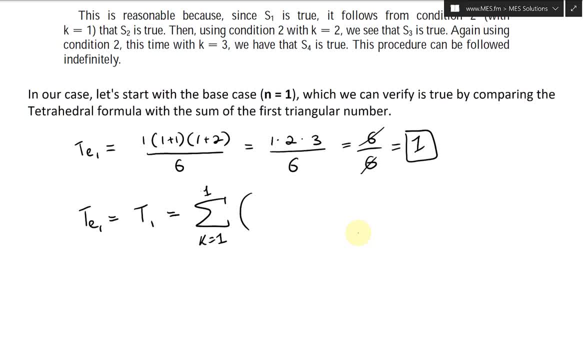 formula here. So this is going to be k times k plus 1, and this is going to be of or actually. just for completeness, let's write the whole thing out: It's going to be up to 1, from actually no up to k. 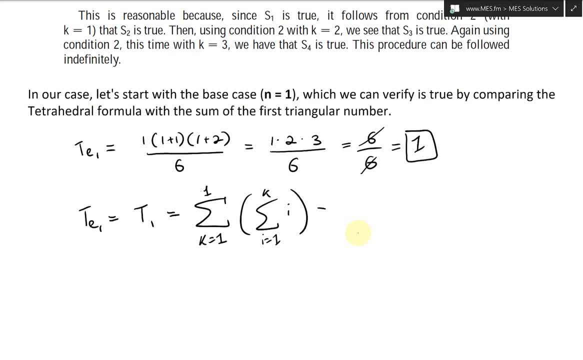 from: i equals to 1, i like that. just for completeness, write this whole thing out and this is going to be up to 1, k equals to 1,. of the formula now: k times k plus k plus 1, divided by 2.. 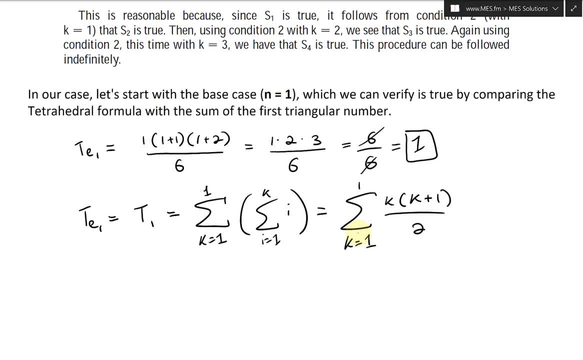 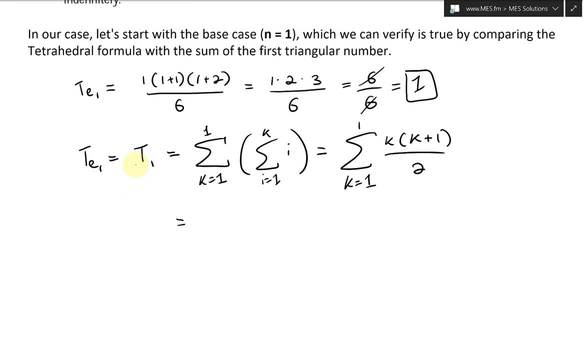 And in other words, this just becomes well 1,. yeah, this is, you just do this once. In other words, just the first triangle. this equals 2, let's put that there for completeness. so this is going to be equals to 1,, which is our k times it by 1 plus 1, which is k plus 1, divided by 2.. 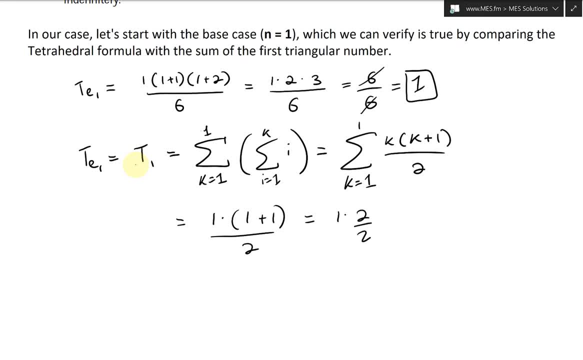 In other words, this becomes 1 times 2 over 2, this cancels equals to 1.. All right, so 1, the base case is true, so this is true, All right. so now that we have, 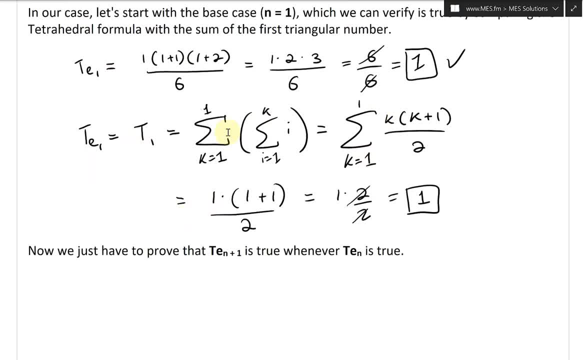 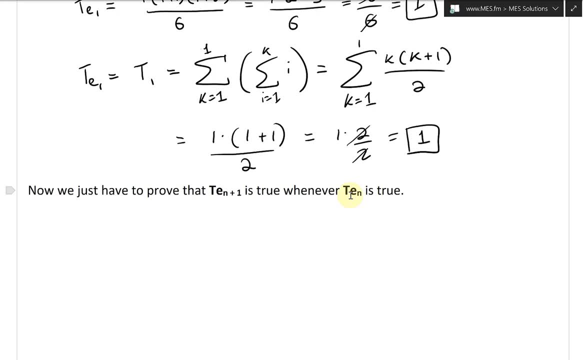 the base case there and I also went a bit overboard just to illustrate how to use this formula. so now we just have to prove tn plus 1 is true whenever t tn is true. So we do the next one here. we've got to prove this. instead of k we'll use n, So we have to prove that this is. 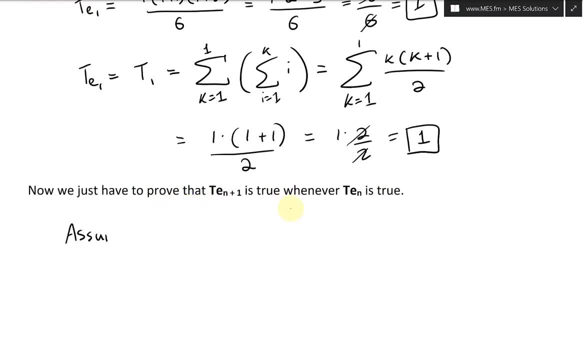 so assume, using induction, assume that t e n is true, So we assume this is true. If it's true, then we're going to have to prove that t e n plus 1 is true. So let's try it now. 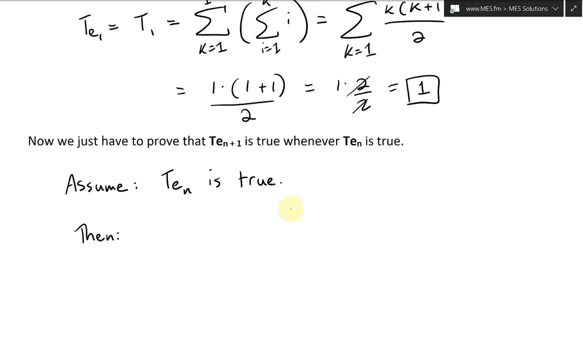 Prove. assume it's the true, then t e n plus 1 is going to equal to. this is going to equal to t e n. so this is the nth, yes, so nth, plus the n plus 1. 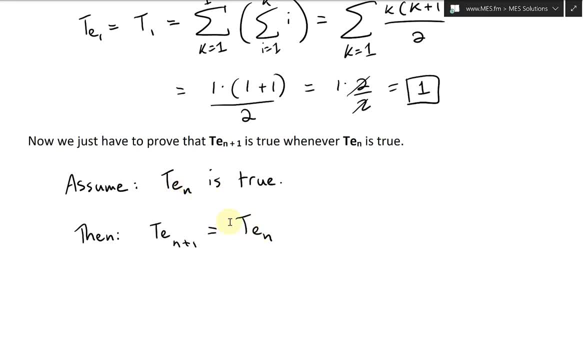 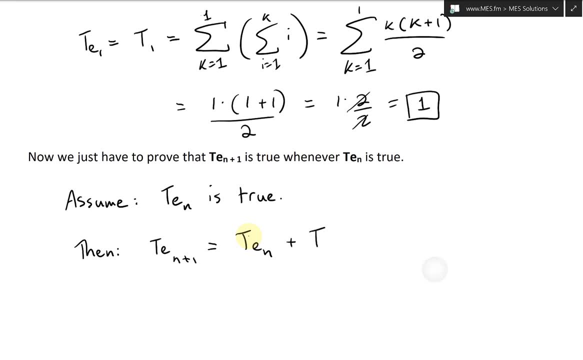 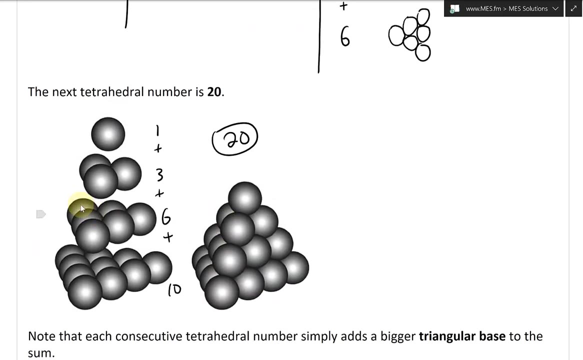 tetrahedral number is equal to the nth tetrahedral number plus the next triangular number, In other words, and then this is going to be plus t and plus one. remember, we're always adding just another triangle number, so that's going to be here. so if we have, in this case, this would be our t, t, n and 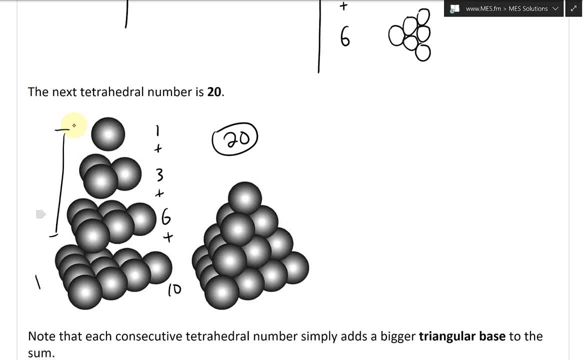 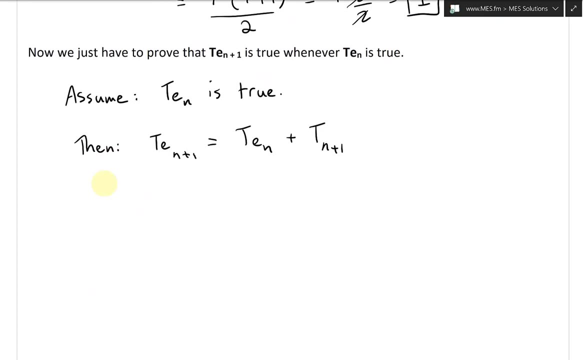 then this next one is this: m. this is t e n. so adding all those together is t e n. then this next one is going to be t and plus one, and then we just add that to it. all right, so this is going to equal two. yeah, this is going to equal two. well, now we have the formula for let's put in the. 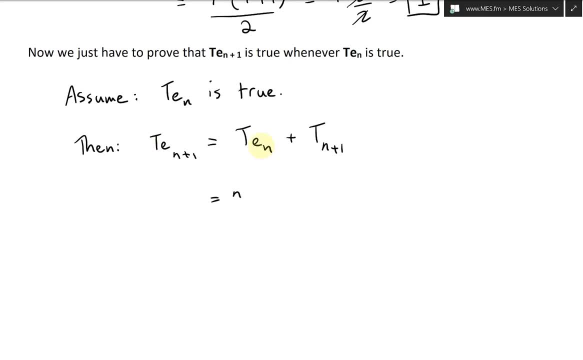 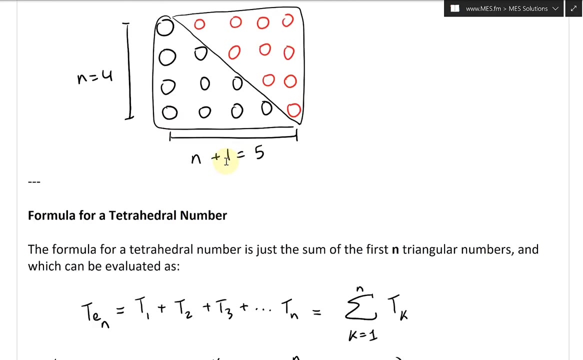 formula for t e a tetrahedral number. that's going to be n times n plus one times n plus two, divided by six plus now, this is the n plus one. uh, a triangle number. so remember, we have the formula for a tetrahedral number and the triangle number is just this, right here. but now we're going to do. 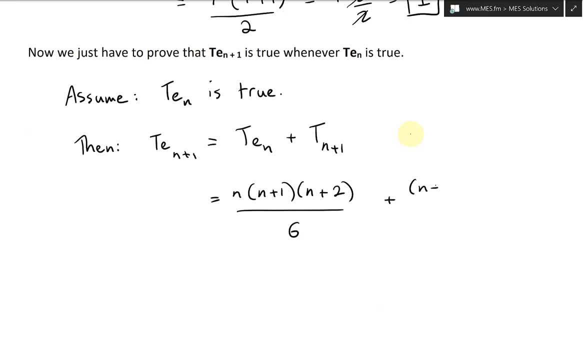 n plus one of that, so that's going to be n plus one times by n plus one plus one. in other words, this is just our n plus two. now, yeah, so this n plus one plus one, this is n plus two. now combine them together. all right, just fix that up. now divide. 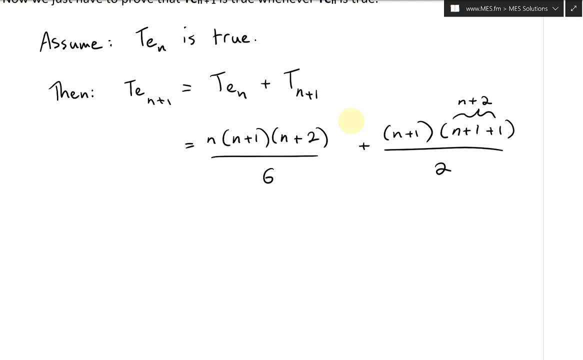 this by two. and now what we could do is, well, we could factor out this n plus two and this whole thing n plus one. so we could factor all that out- this equals to n plus one- and factor n plus two out as well, and then what we're left with is now this n plus n divided by six, and then we just have, well, one. 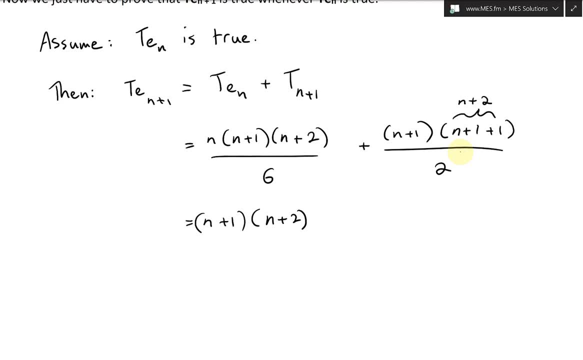 divided by six there, because we factor out the whole thing there and then times this by a big bracket like that- n over six plus one over two, like that- and then what we could do now is: well, we have this bracket. i'm going to do now is multiply the top and bottom of this one by 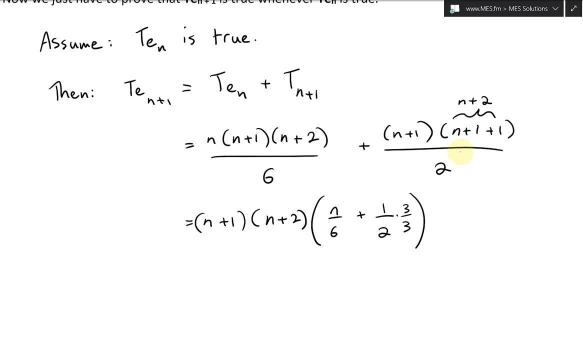 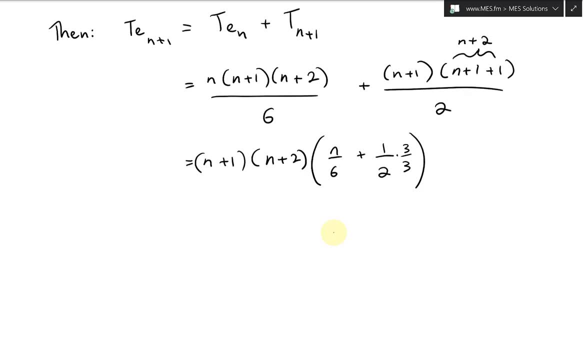 three over three, it's three times uh divided by three. so that doesn't change anything, but we're gonna have the same common denominator, six, there. so this equals to n plus one, n plus two, and now what we have here is n plus three divided by six. so in other words, we got our formula it's gonna be. now let's put this like this: 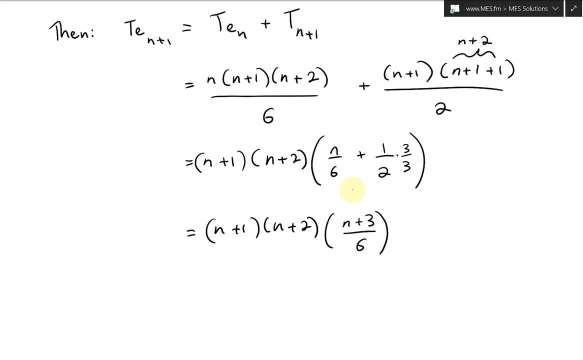 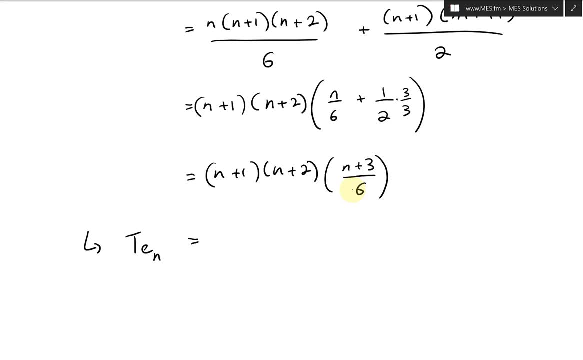 n plus three divided by six, and that is our formula, and let's put it all in the format. we're but an arrow: t e, n plus one is equal to two. yeah, this is actually yeah. this is n plus one of it, though: n plus one, n plus two, n plus. 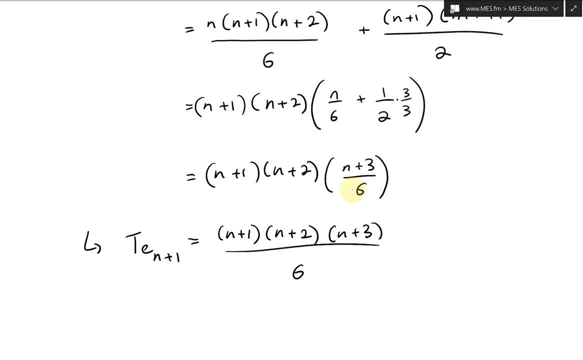 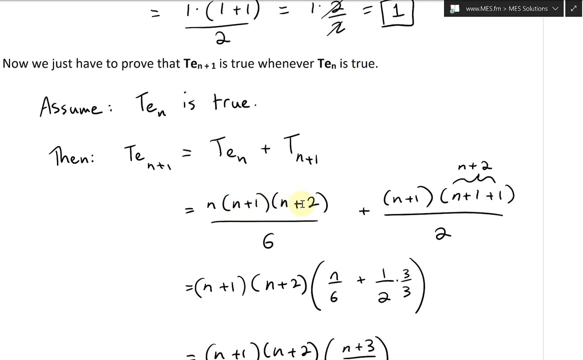 three all divided by six, and in other words: uh, this, right here, this is true. this means it's: uh, that formula is true because, well, we know tn, assume that it's true. and tn is just n plus one, n times n plus one, times n plus two. but now we're replacing with n plus one, so n plus one. 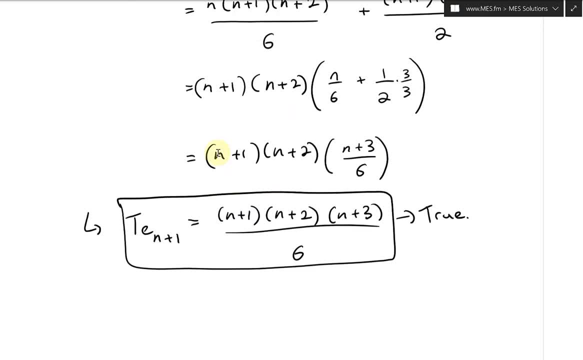 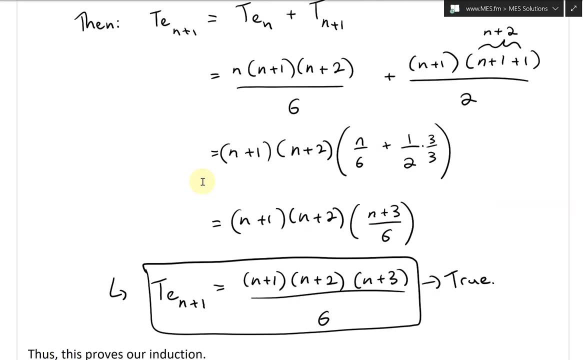 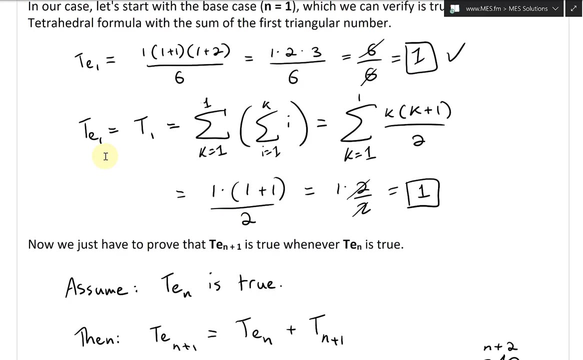 then it's gonna be n plus two and plus three. so that's true. thus we've proven our uh formula. yeah, and thus this proves our induction, because, well, tn, te, n plus one is true, uh, whenever t, e, uh, nth, yeah, tn is true and we know that the base case is true. so then t2 is true, te2 is true, t3, etc. 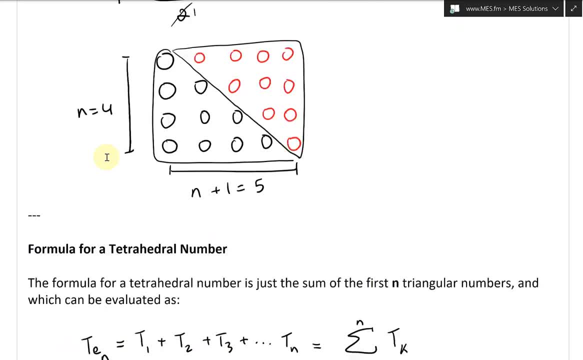 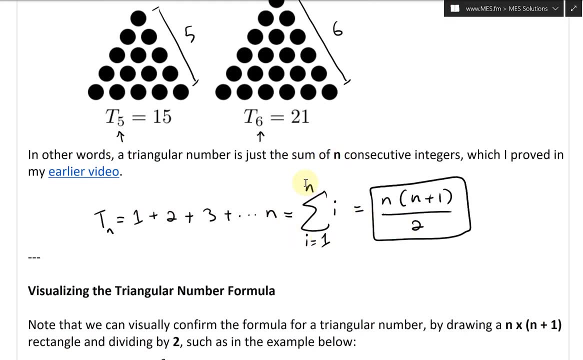 and going there's. that's all for today. i hope you enjoyed. this video is a bit extensive. i just had to cover the triangle numbers. i didn't cover those before and yeah, those are the just the sum of n consecutive numbers which i had shown in my earlier video. that proof equals to: